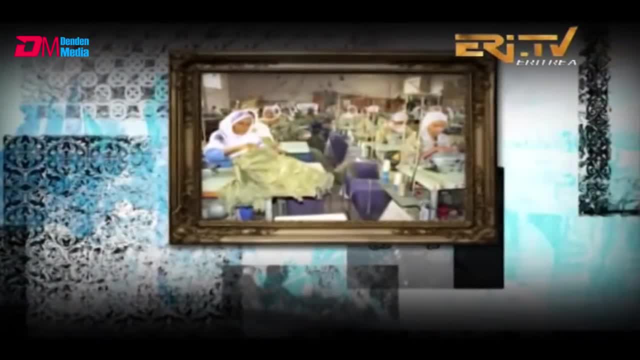 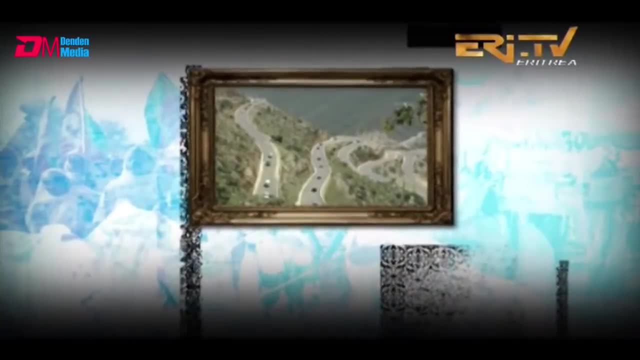 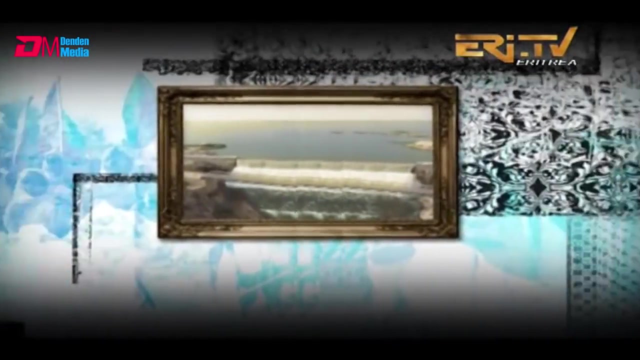 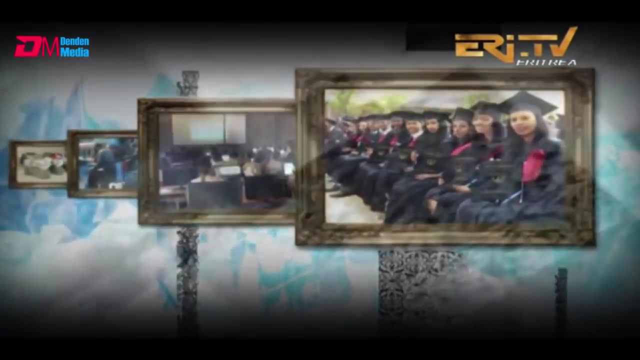 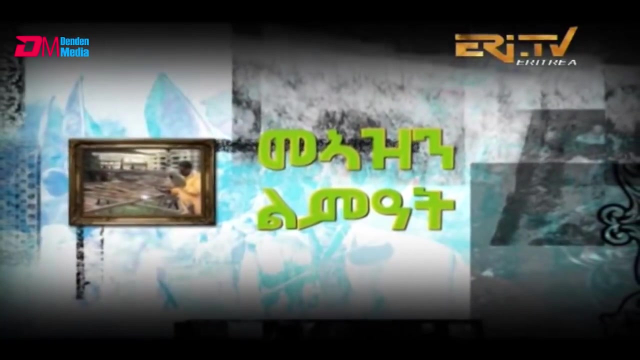 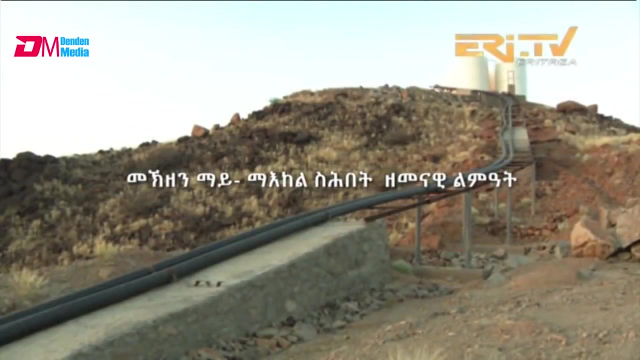 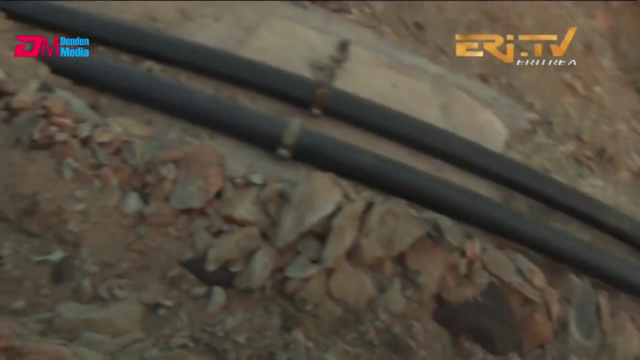 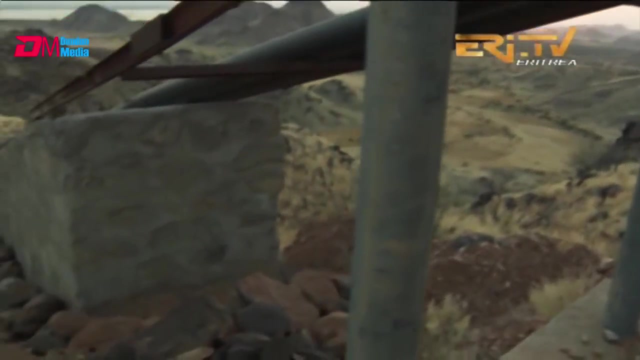 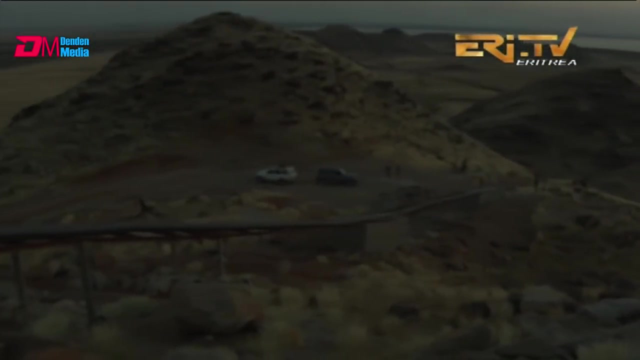 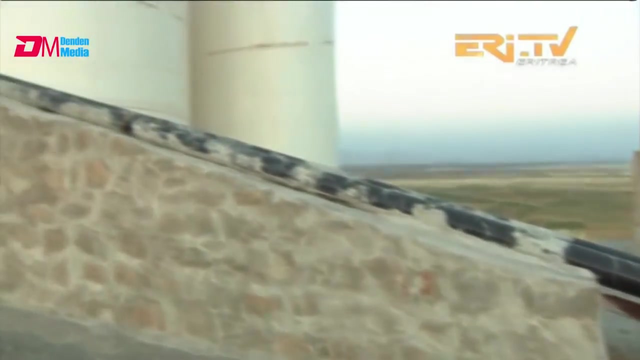 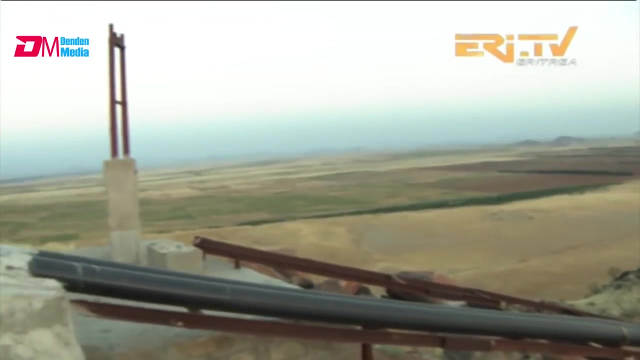 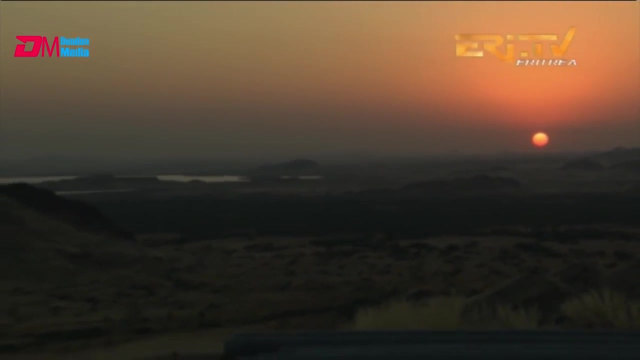 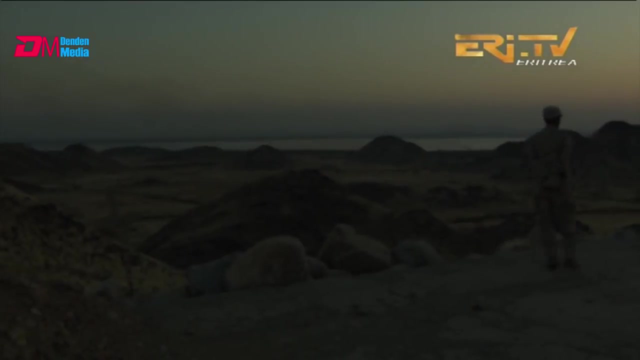 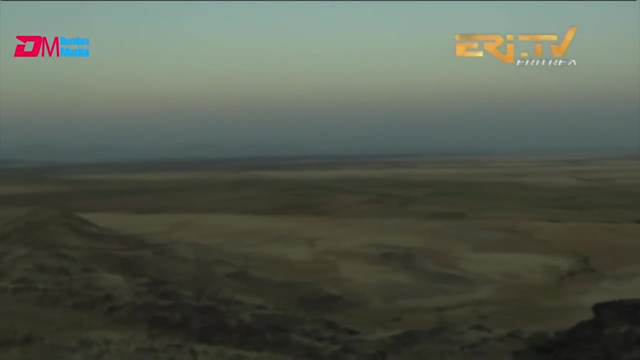 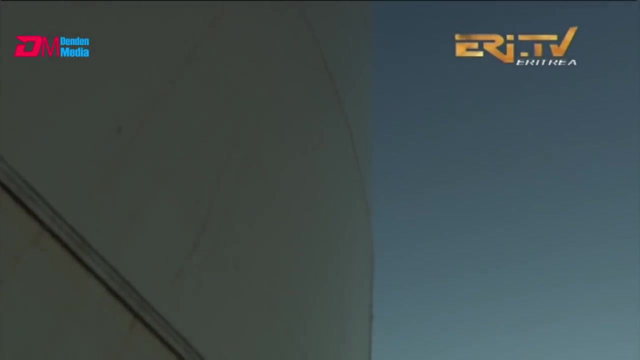 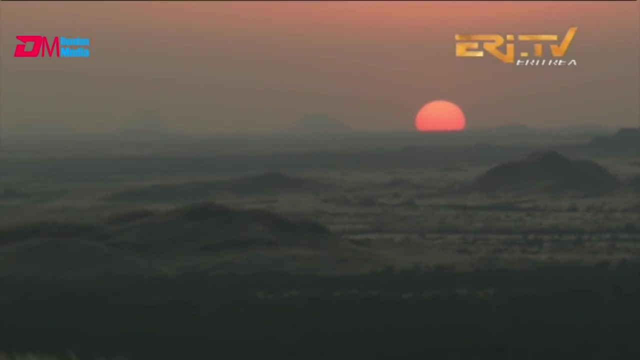 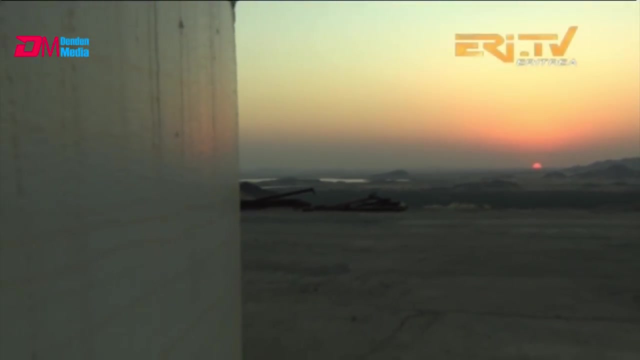 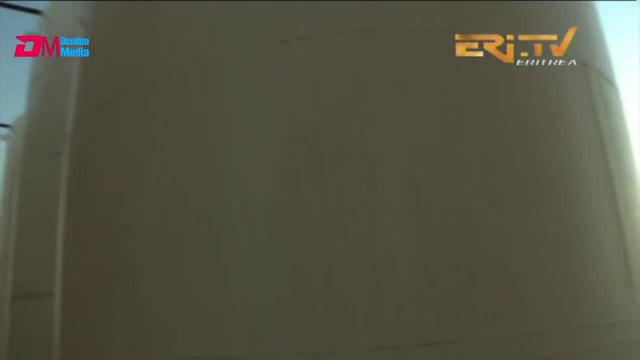 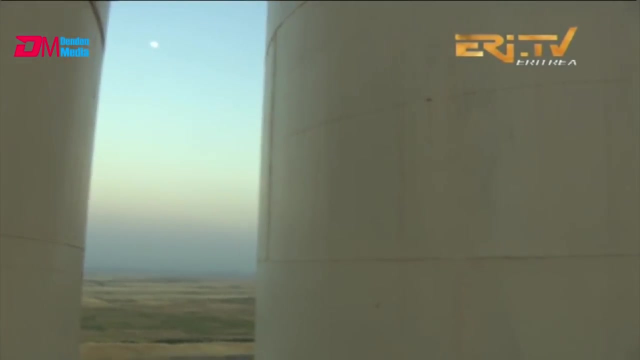 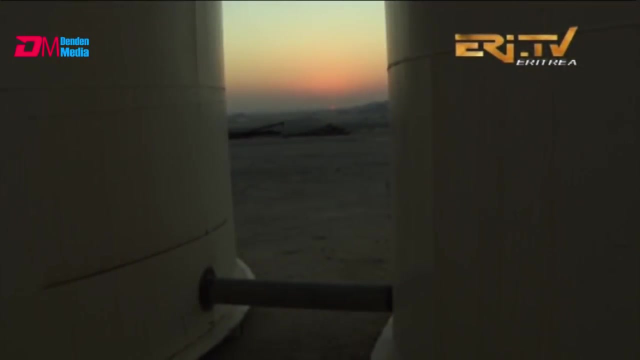 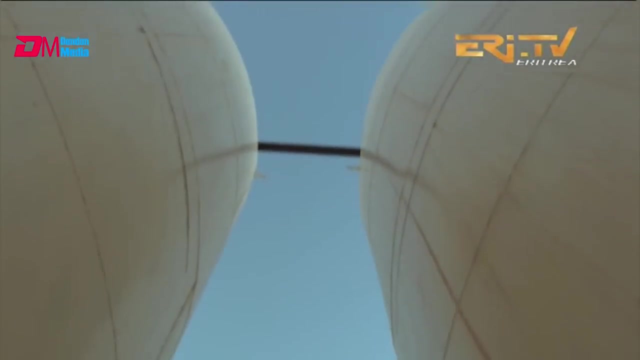 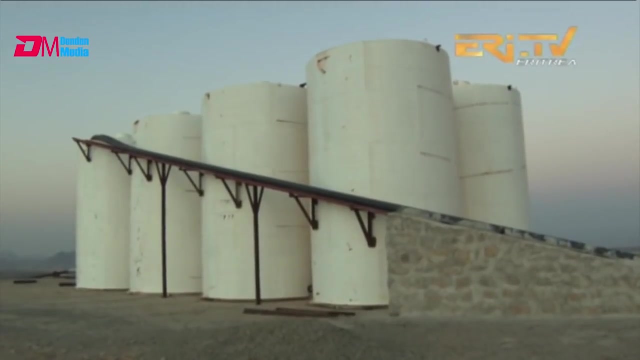 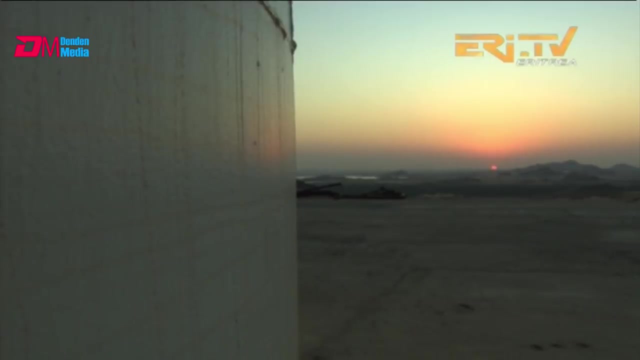 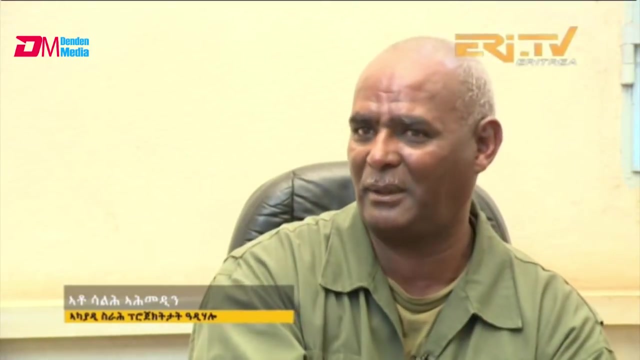 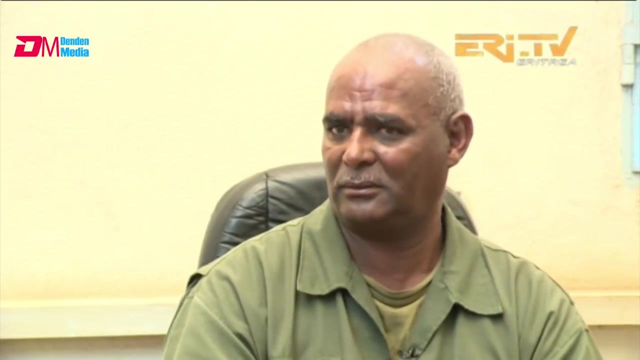 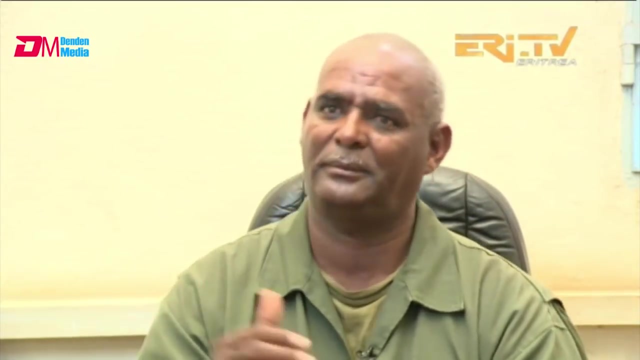 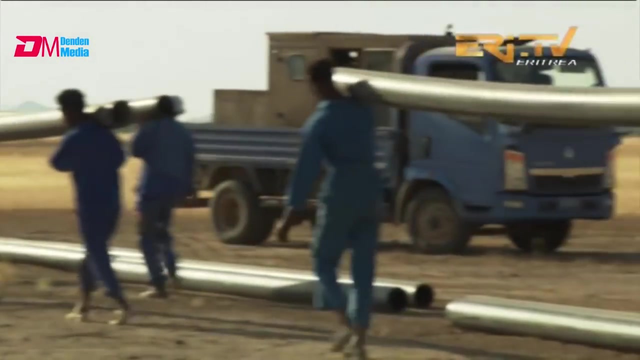 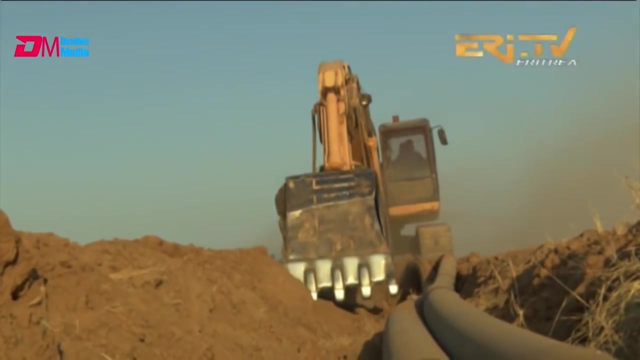 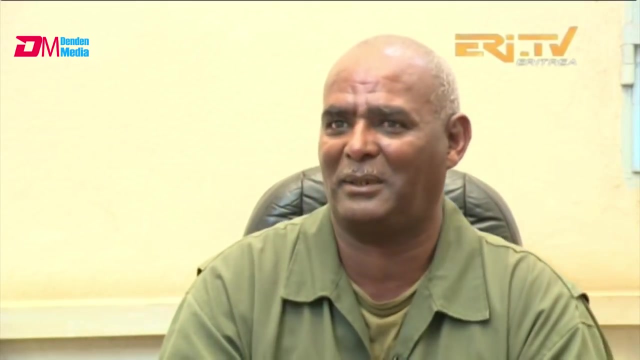 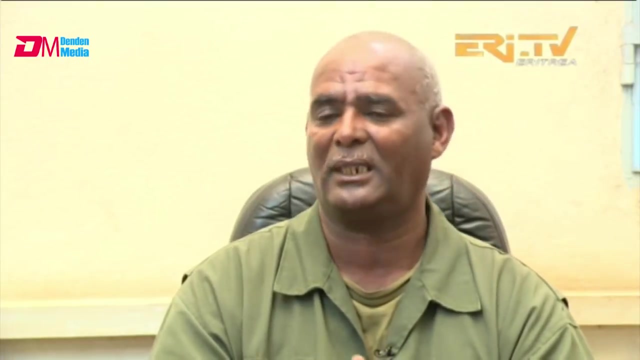 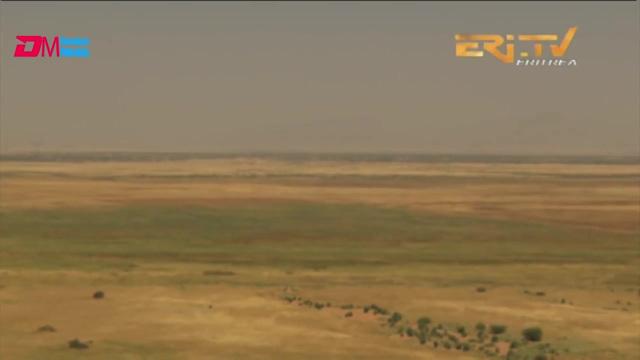 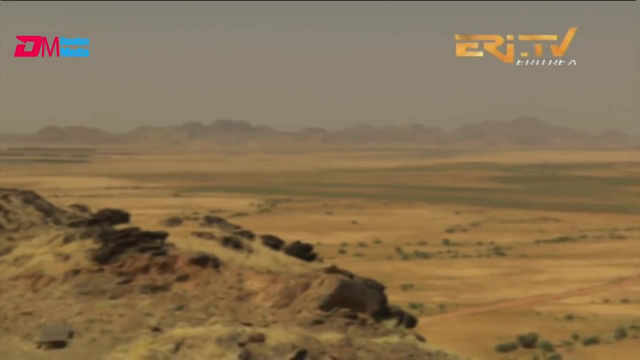 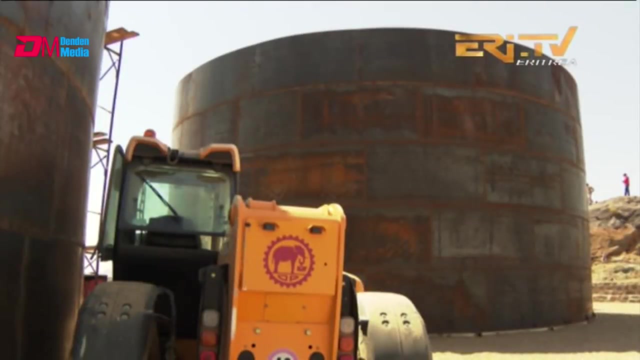 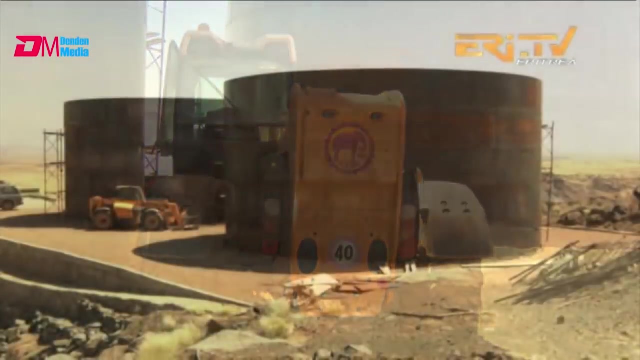 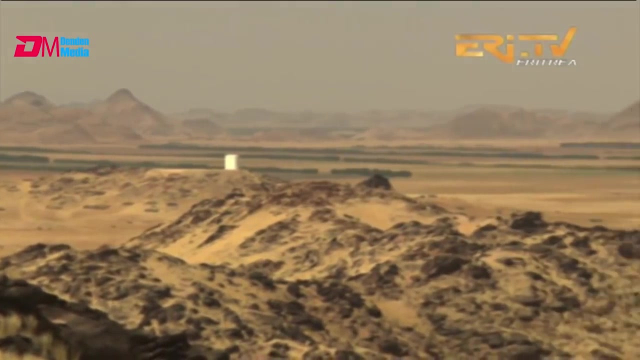 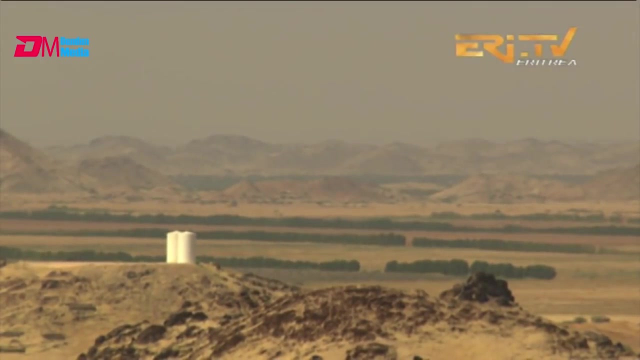 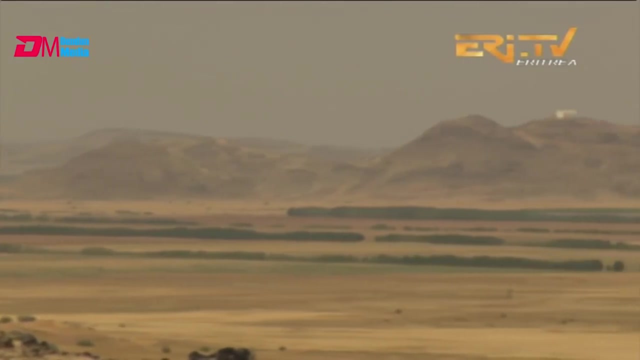 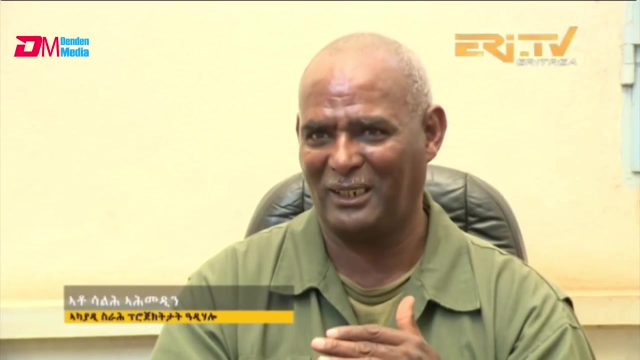 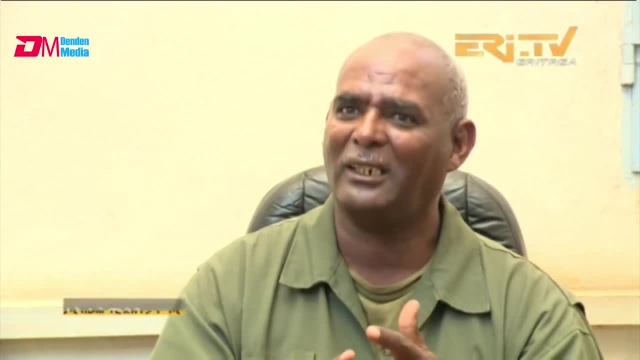 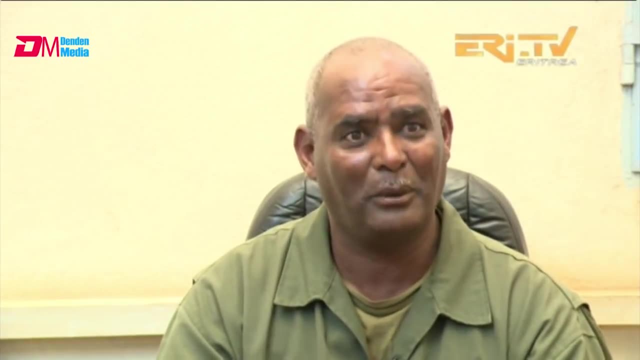 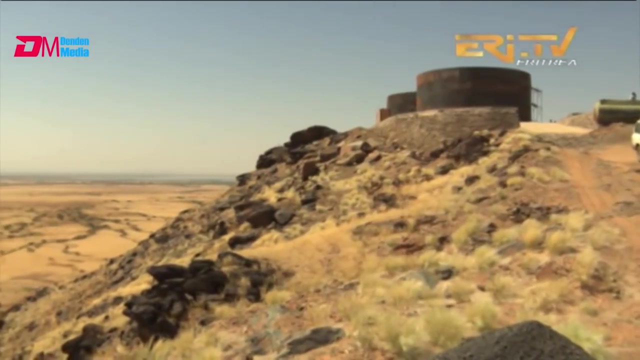 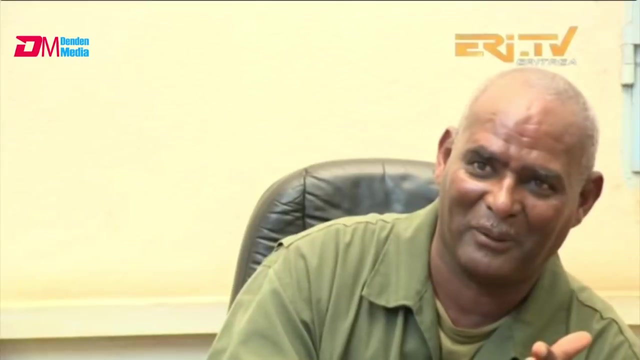 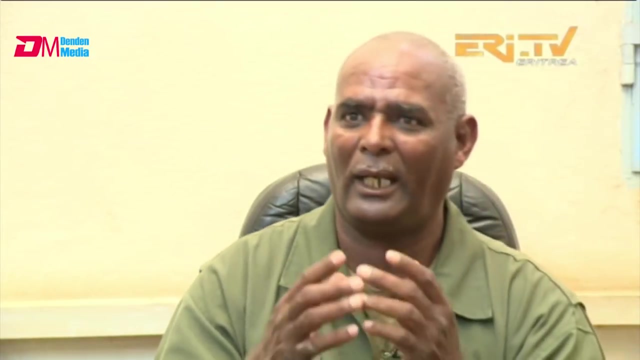 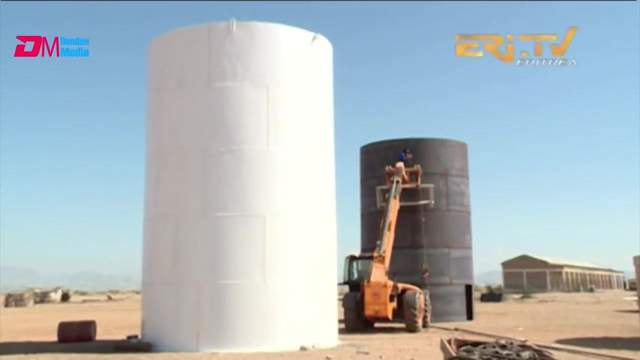 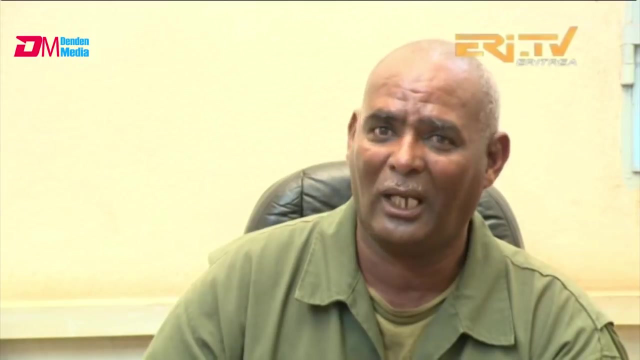 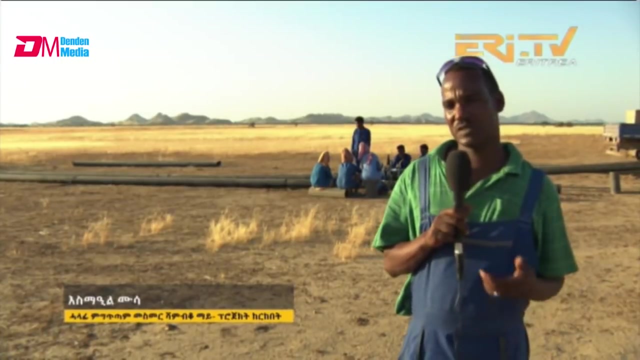 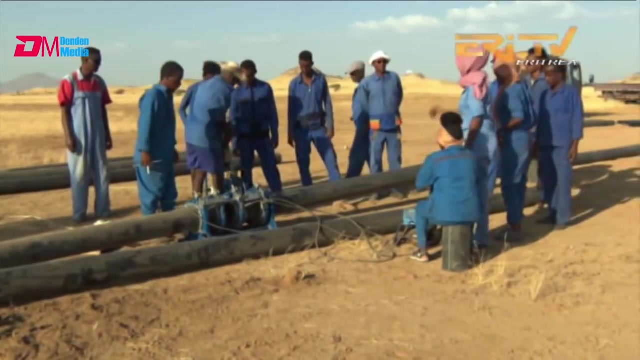 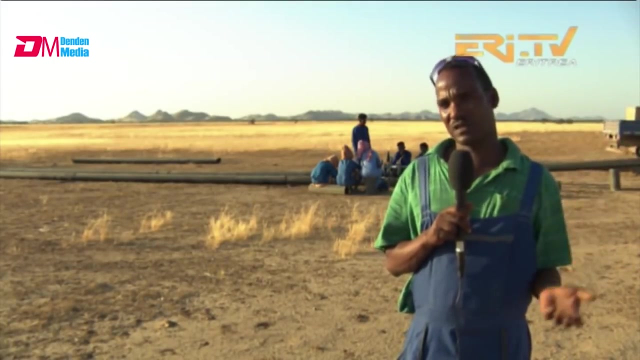 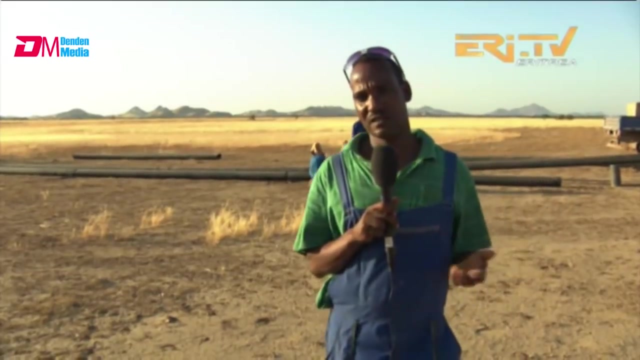 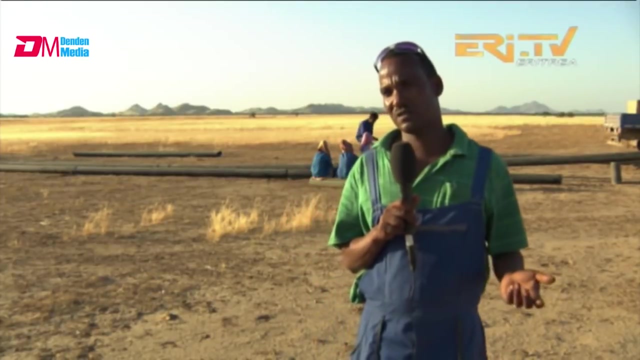 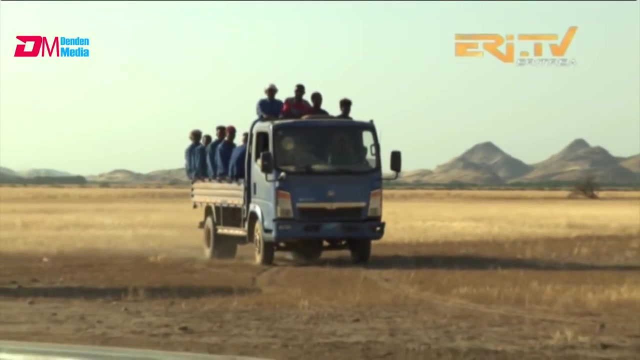 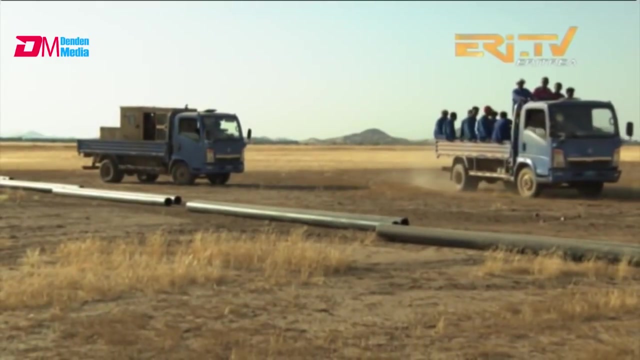 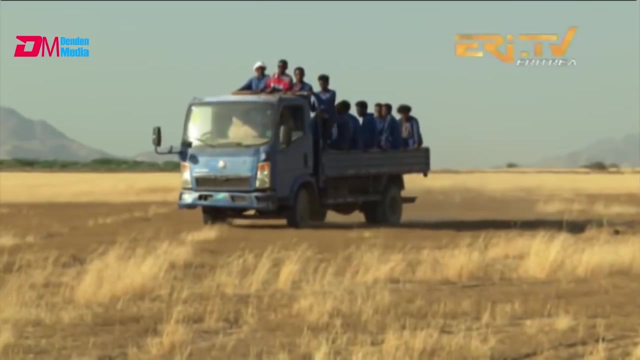 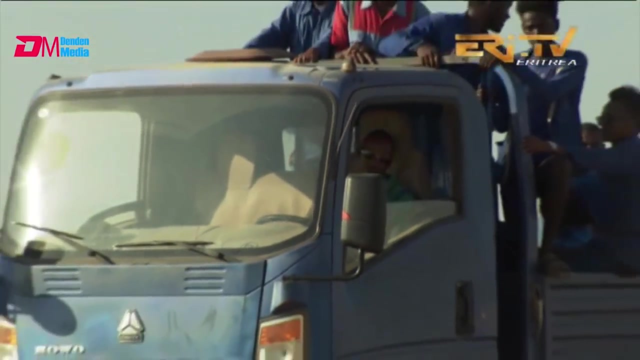 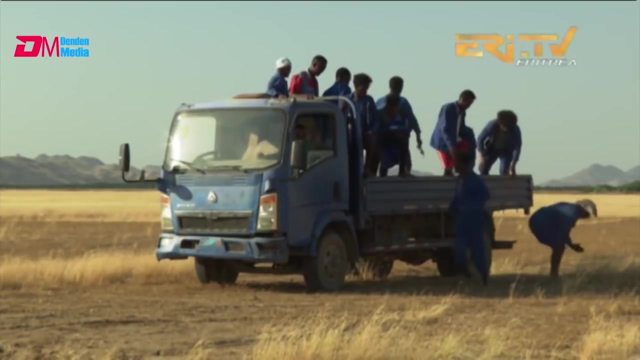 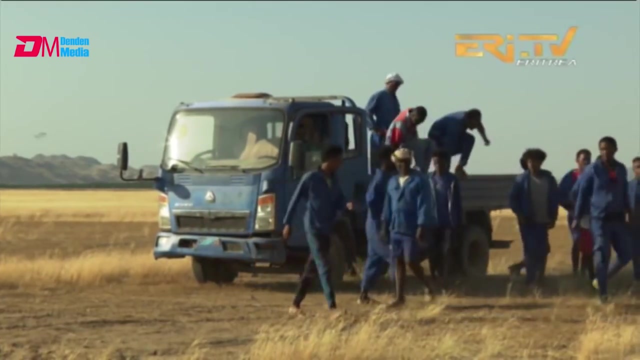 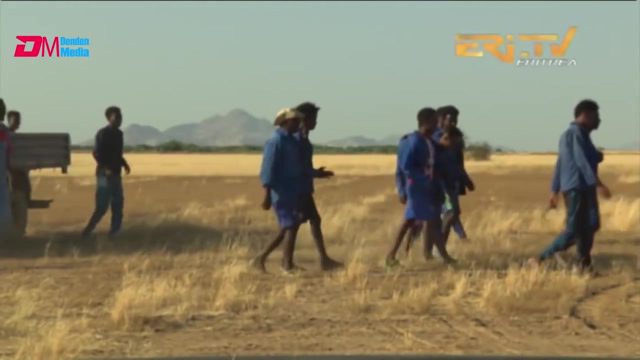 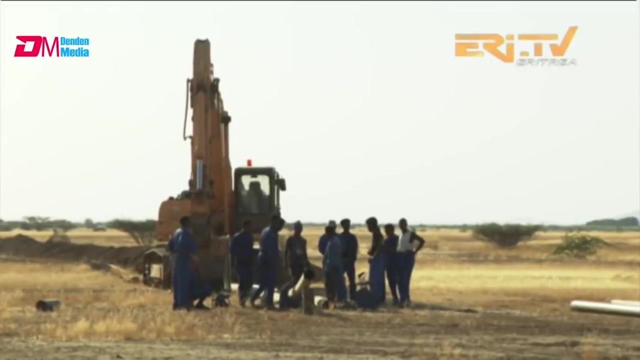 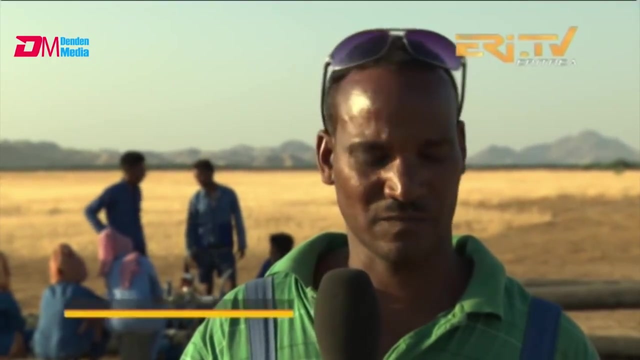 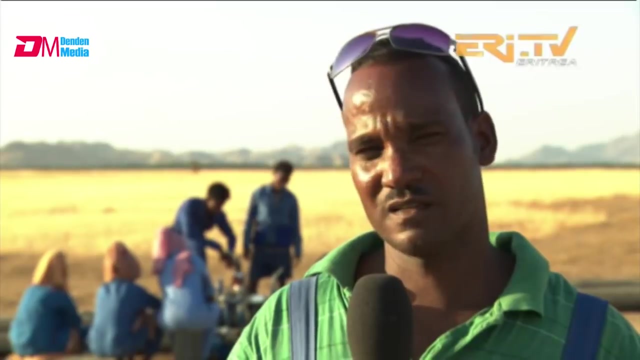 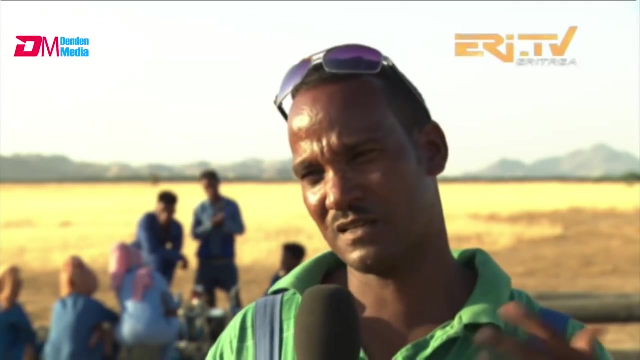 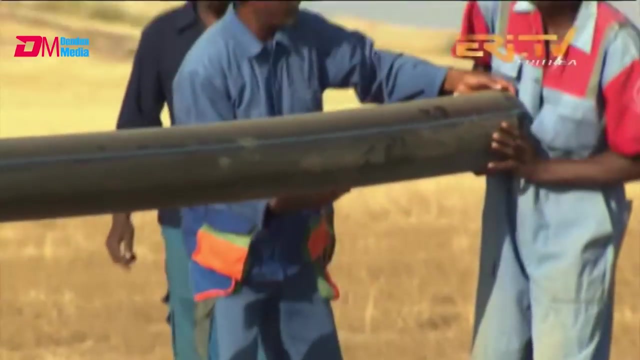 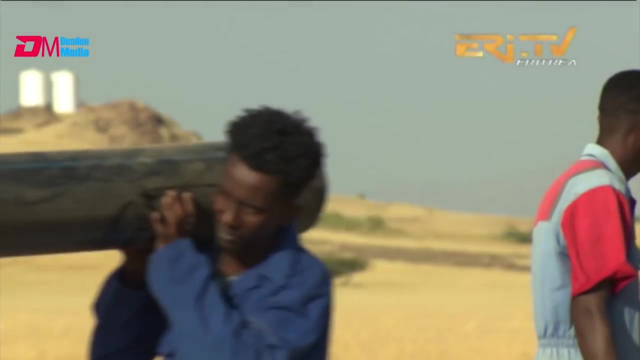 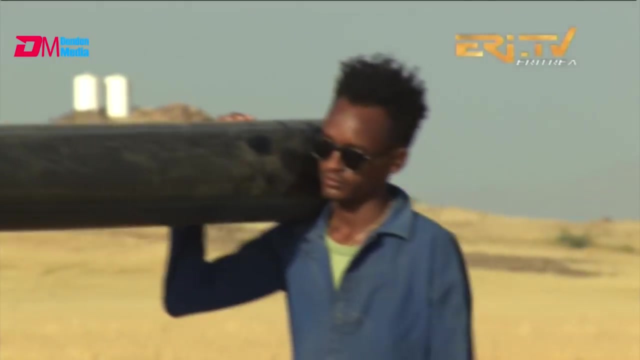 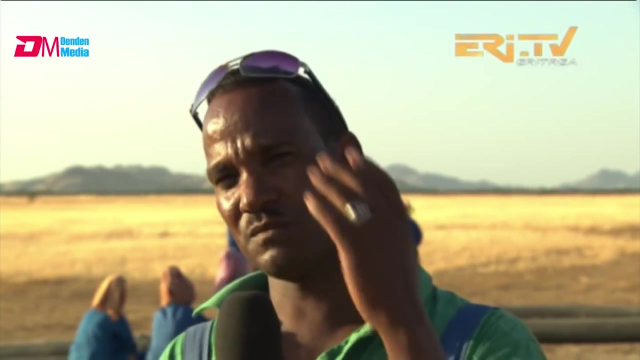 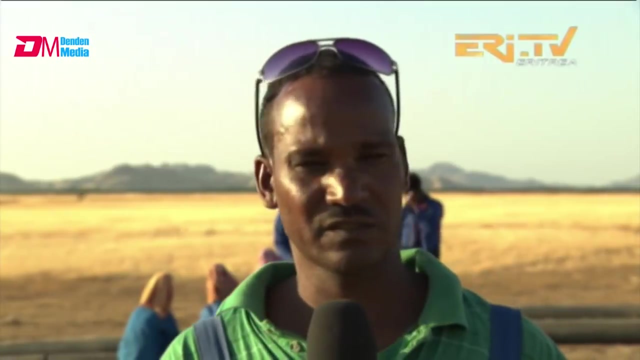 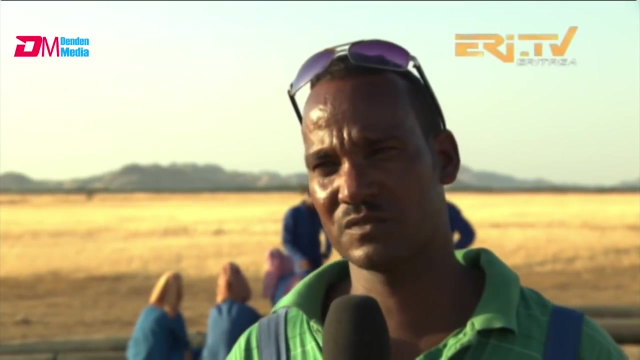 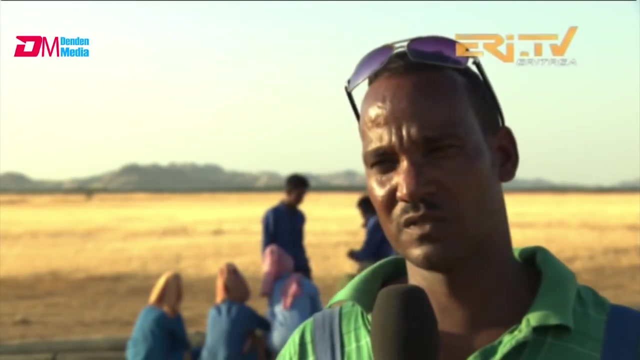 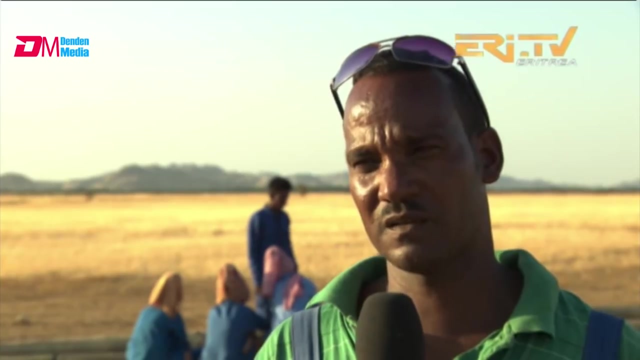 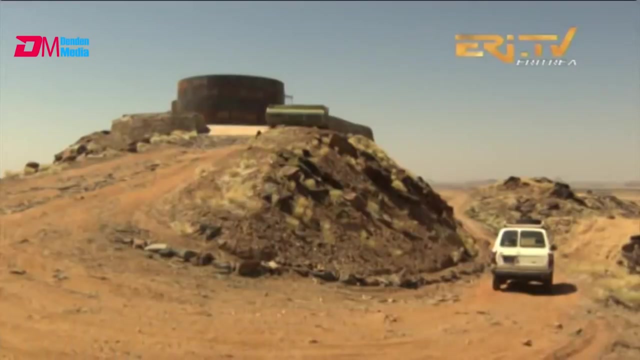 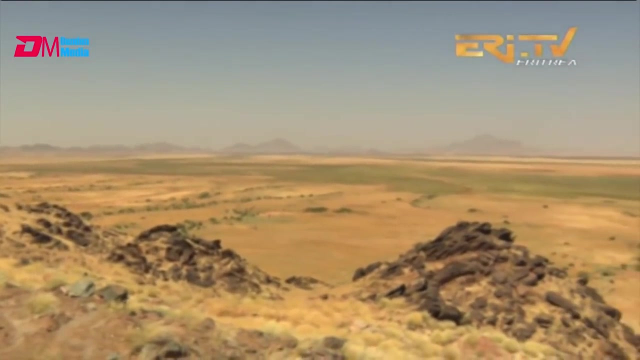 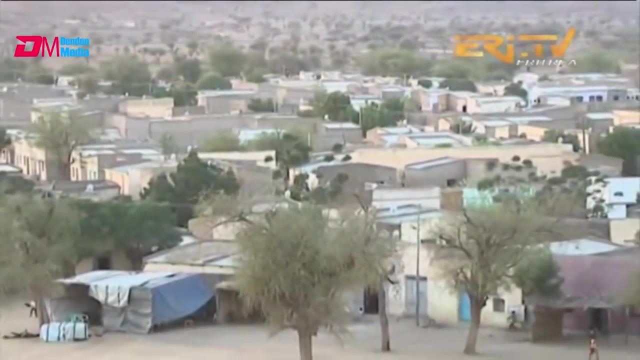 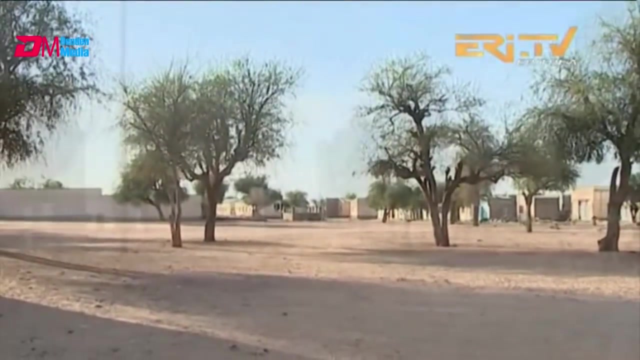 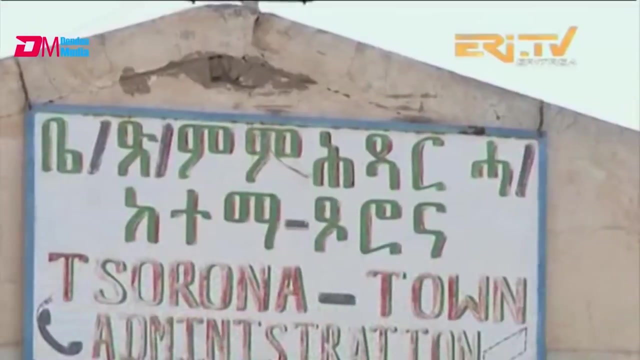 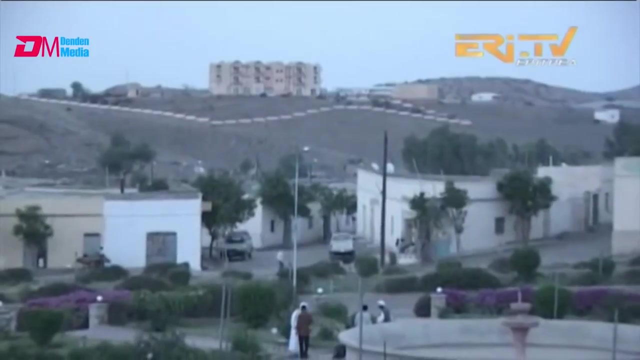 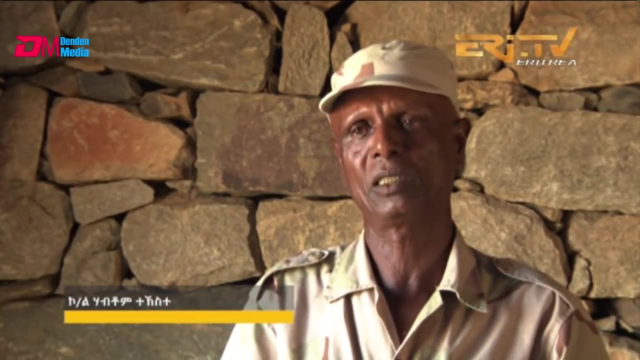 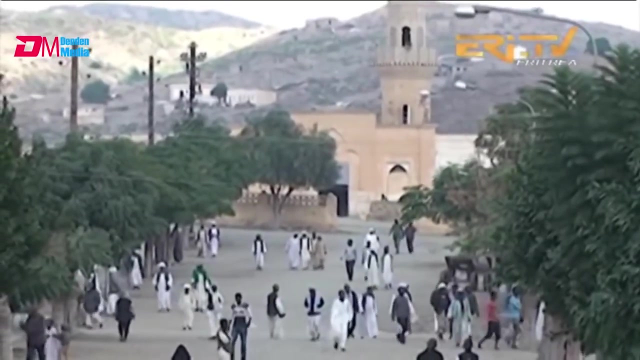 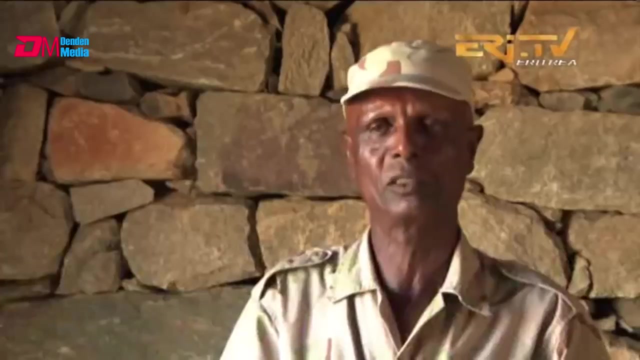 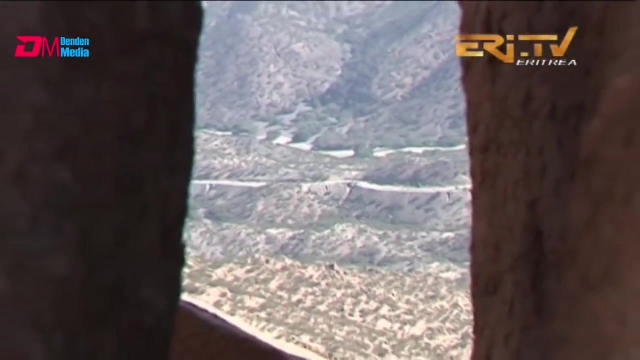 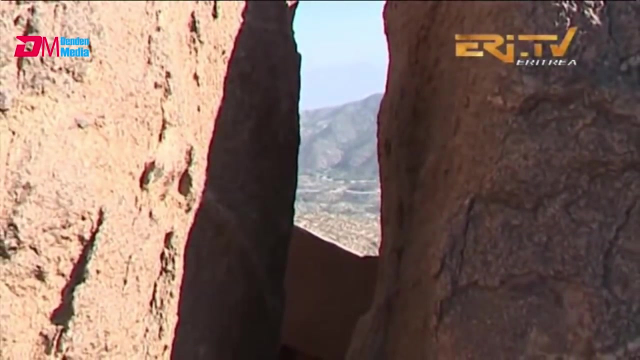 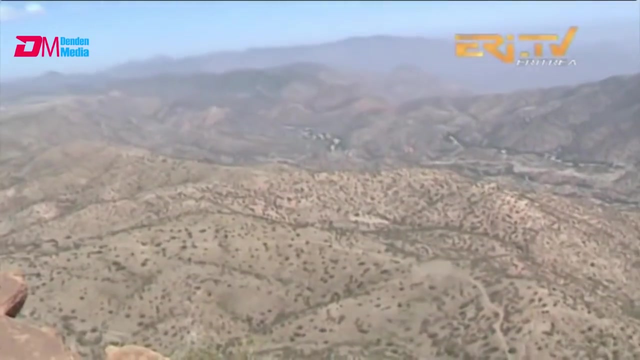 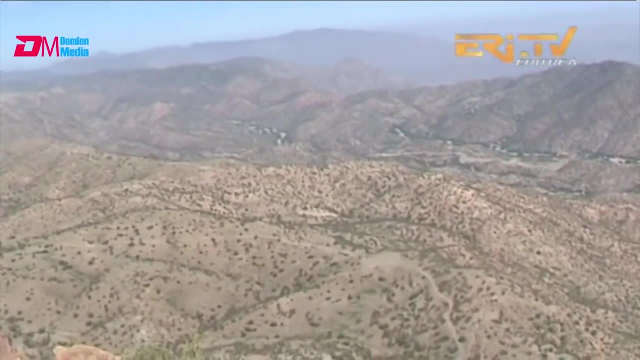 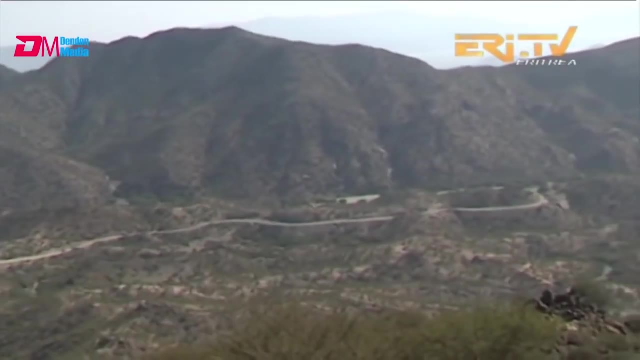 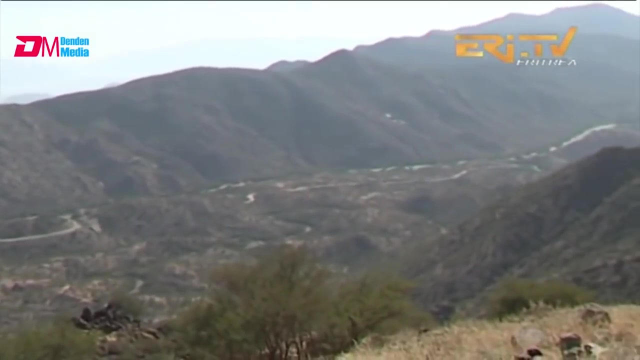 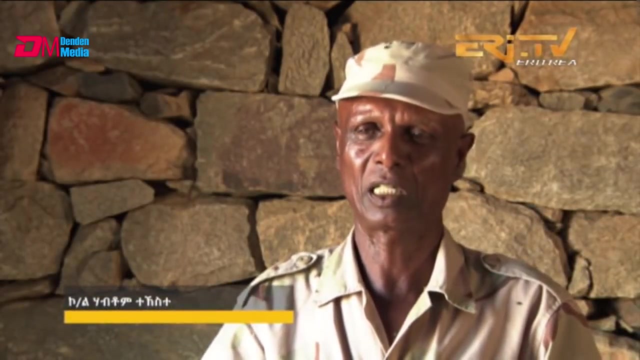 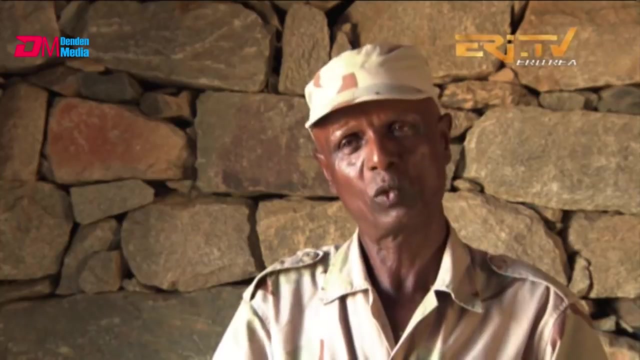 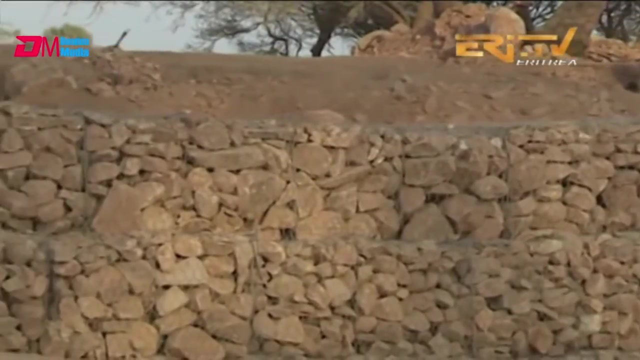 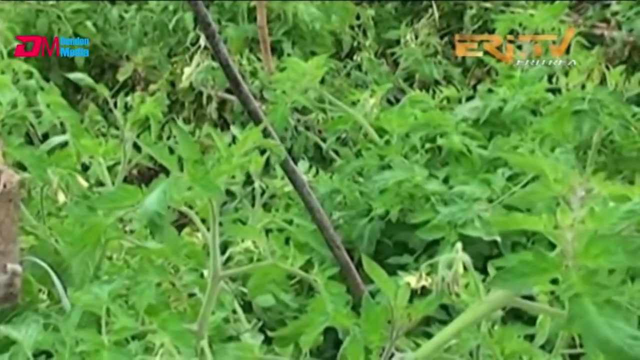 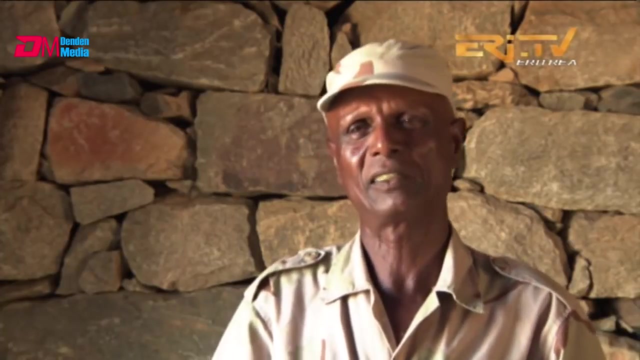 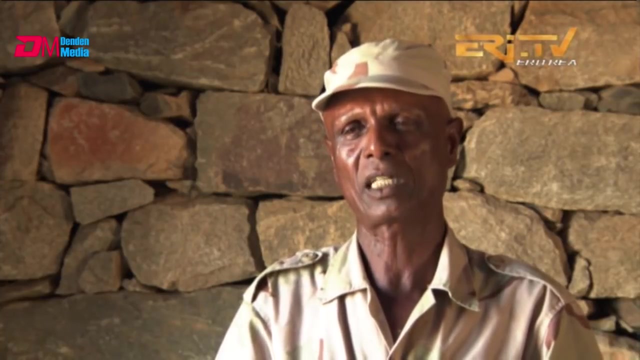 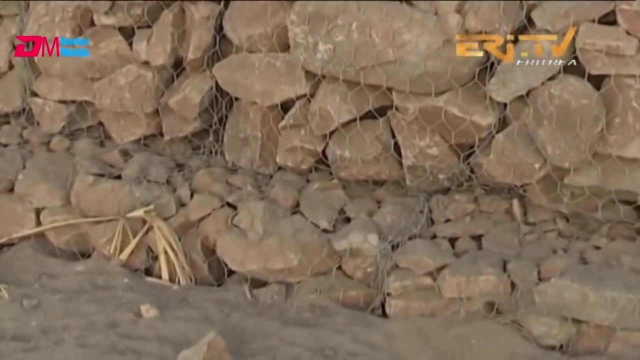 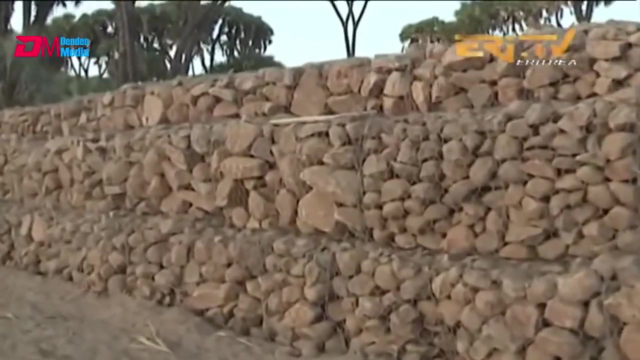 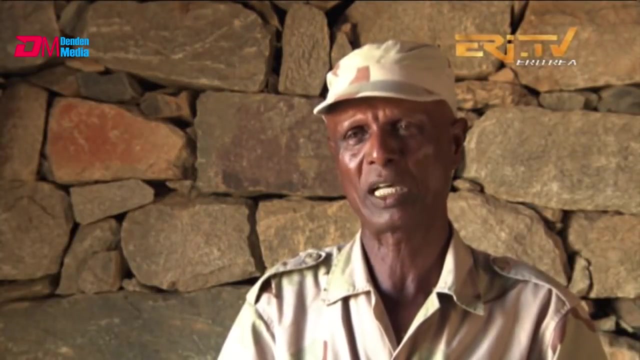 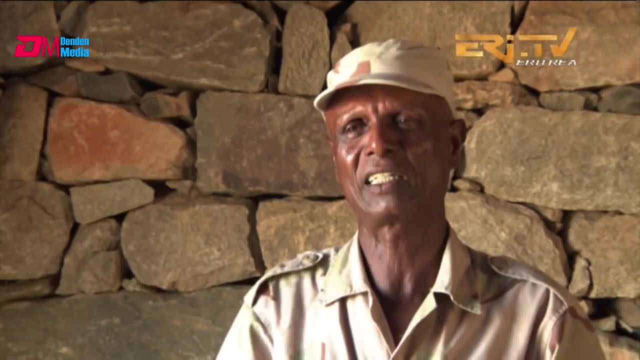 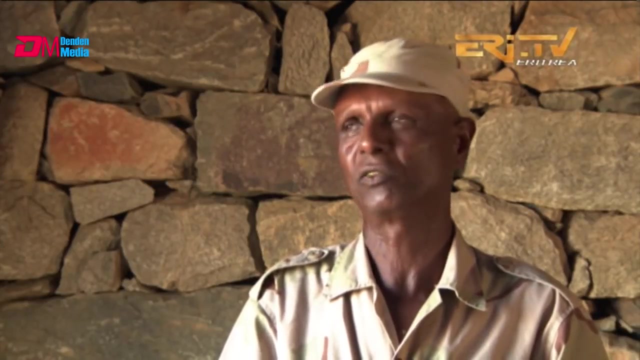 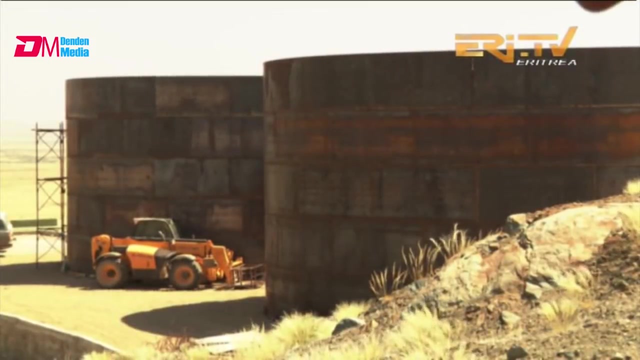 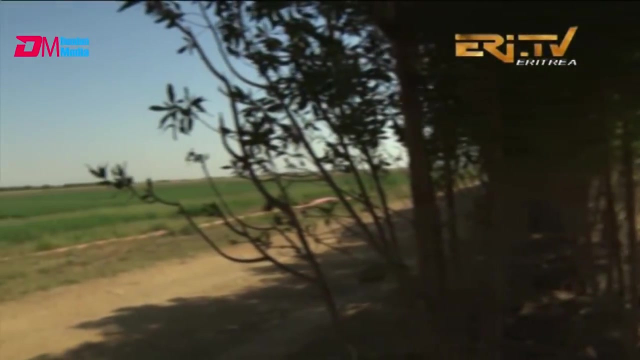 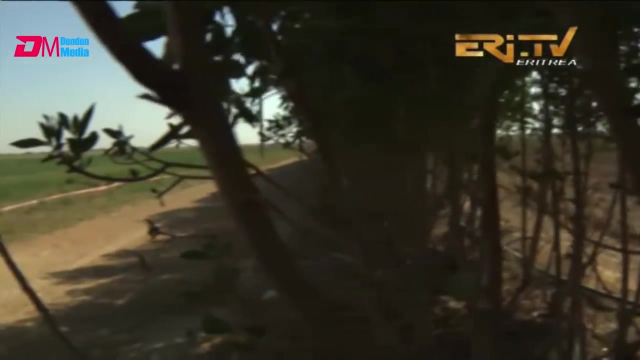 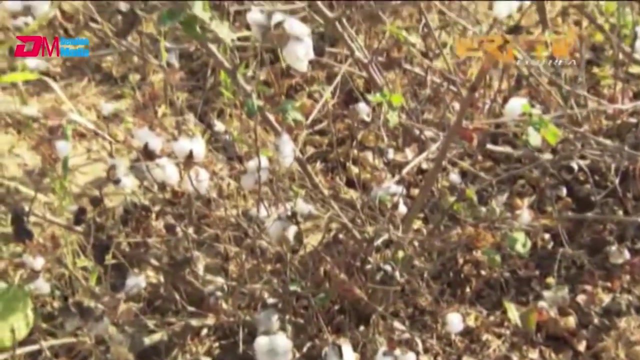 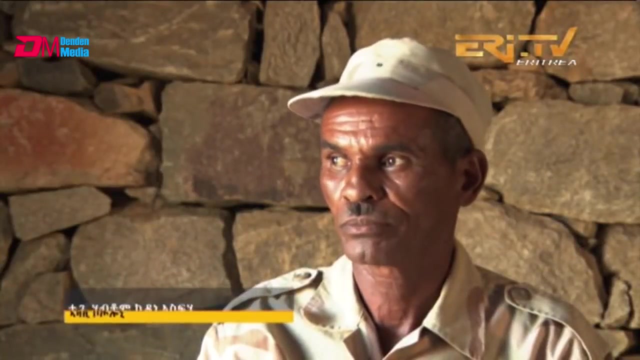 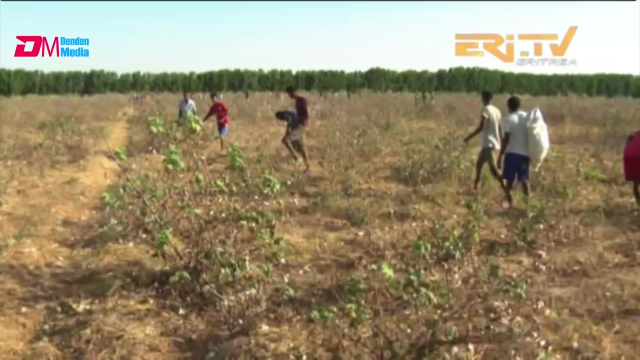 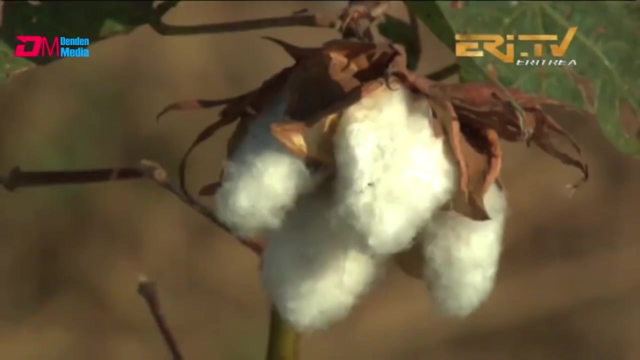 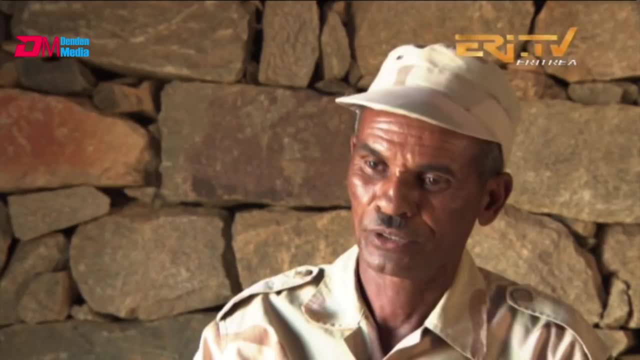 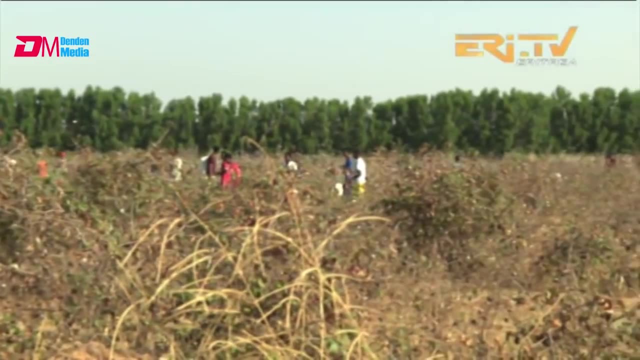 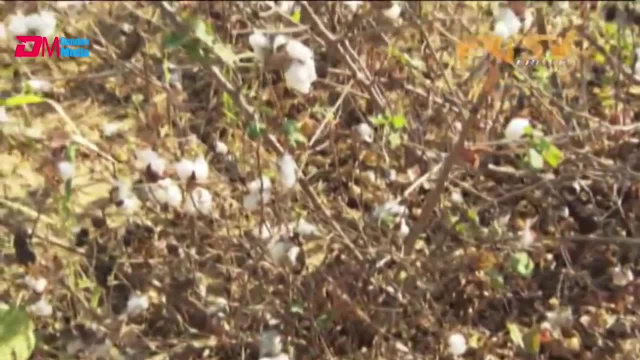 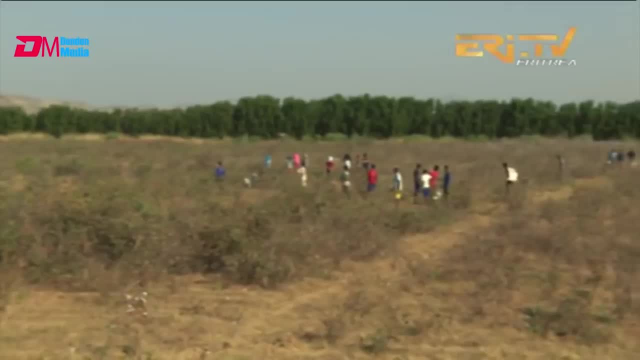 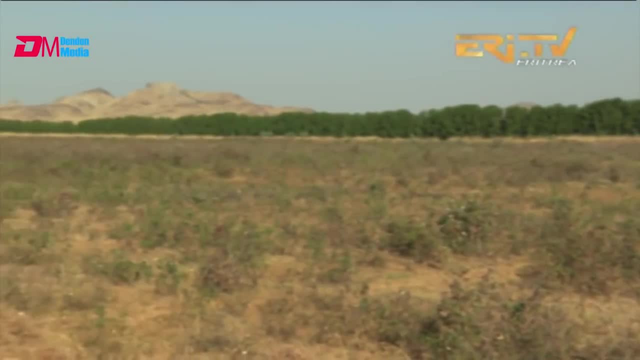 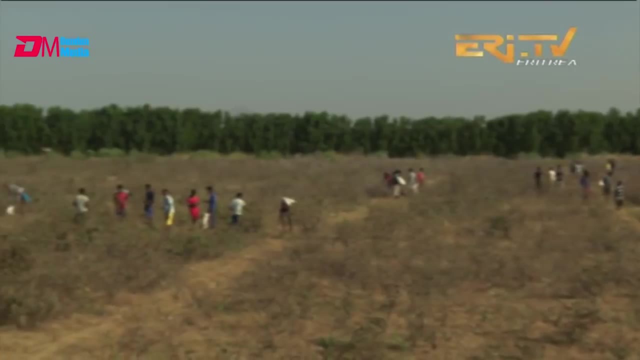 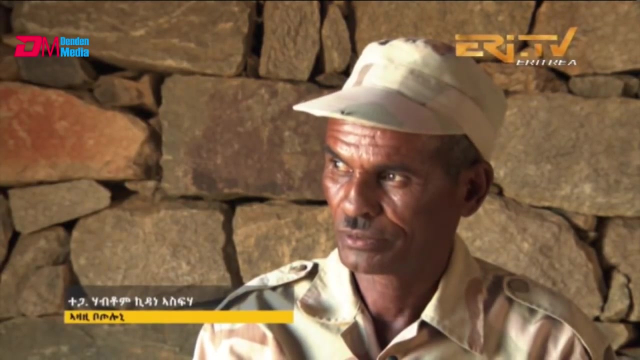 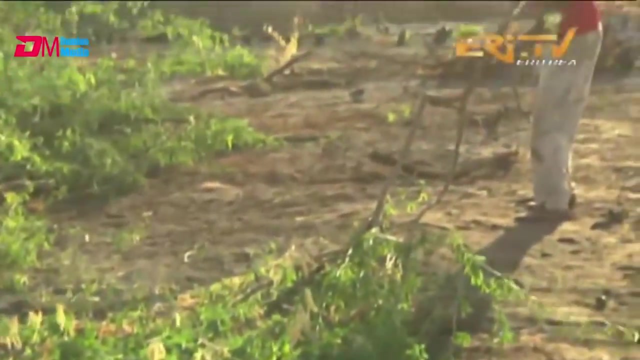 Thank you for watching. Thank you for watching. Thank you for watching. He says he is very happy to be able to share his knowledge and experience with us. I am very happy to be able to share my knowledge and experience with you all. I was able to make a living by selling things. 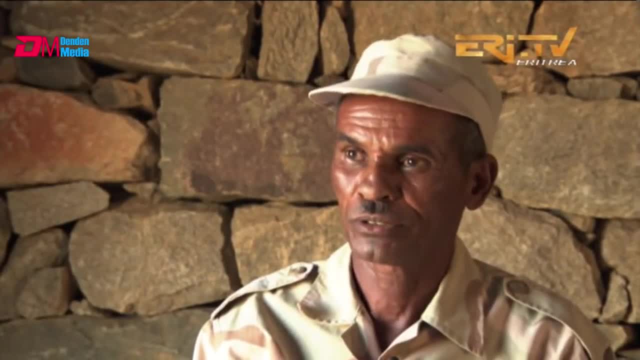 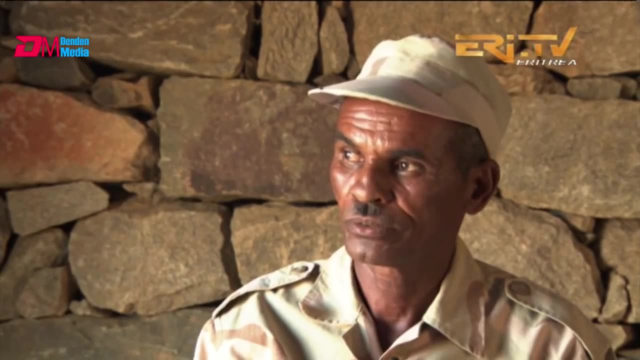 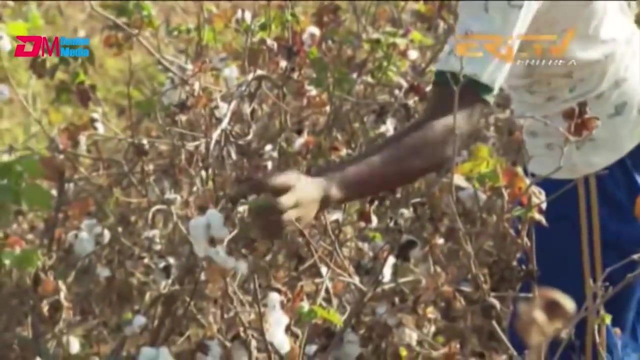 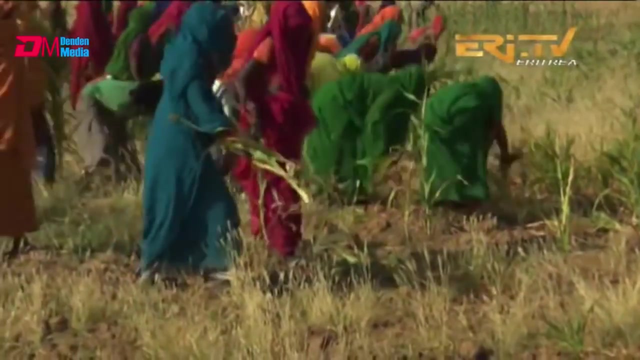 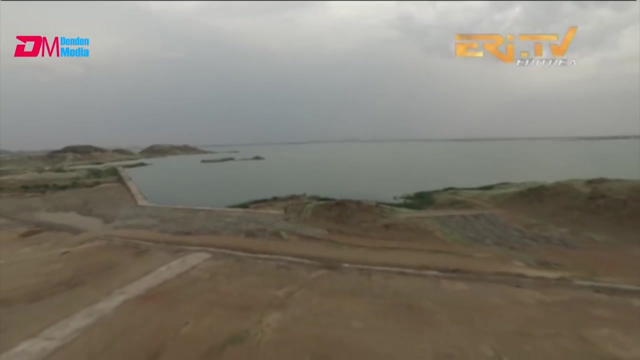 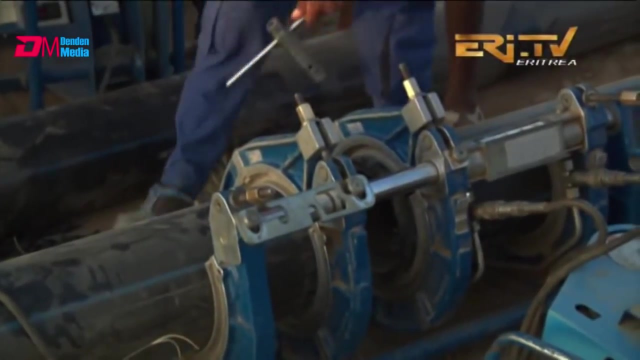 I also have a business. I work in the factory in the village of Birkayou. I have a business there. The project is part of the project, which is part of the project, which is part of the project. We are in our fourth week of Covid-19.. 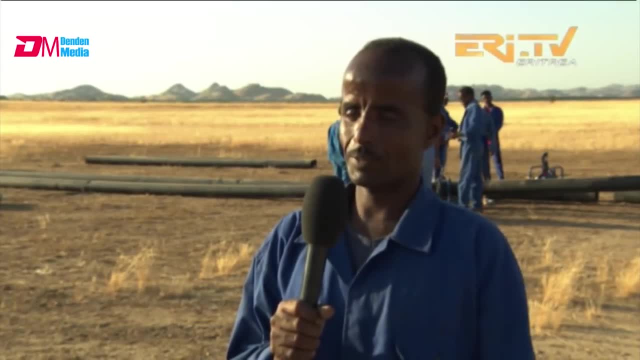 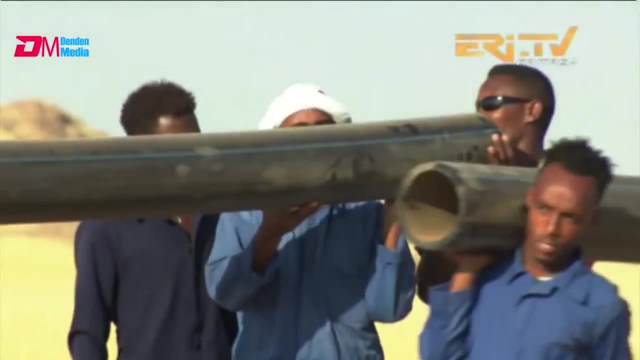 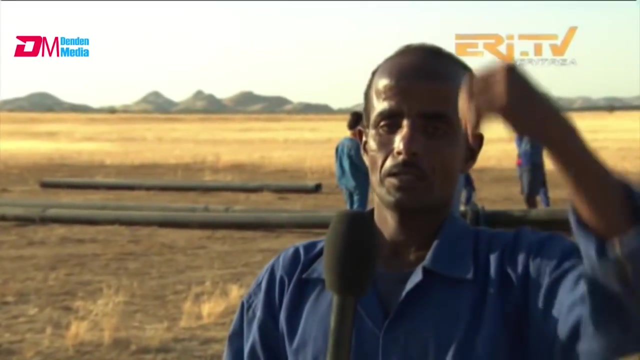 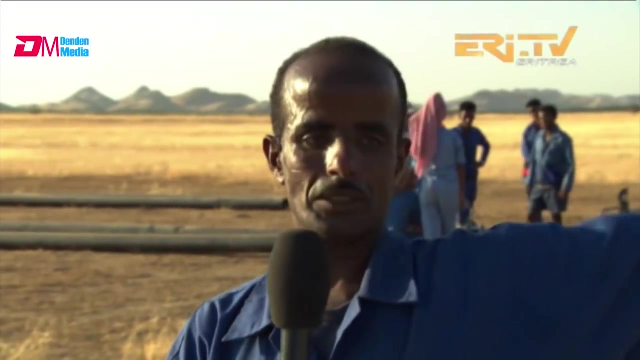 We have been in lockdown since the start of the pandemic. We have been in lockdown for one month. We are in lockdown and we are trying to maintain the order. I have been working here for almost a year and a half. I hope to return here in the future. 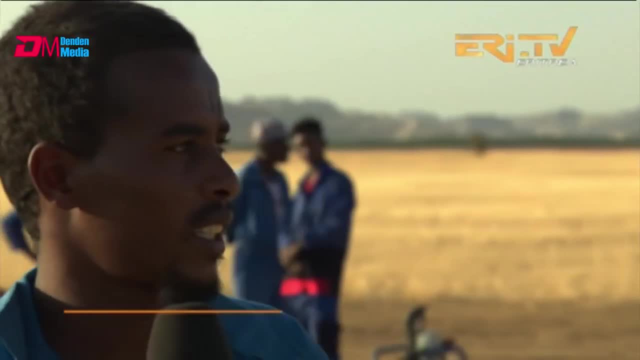 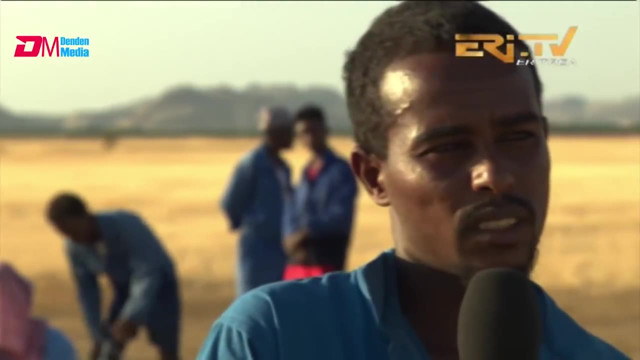 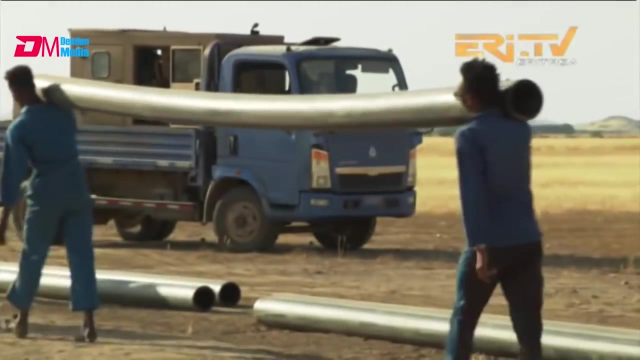 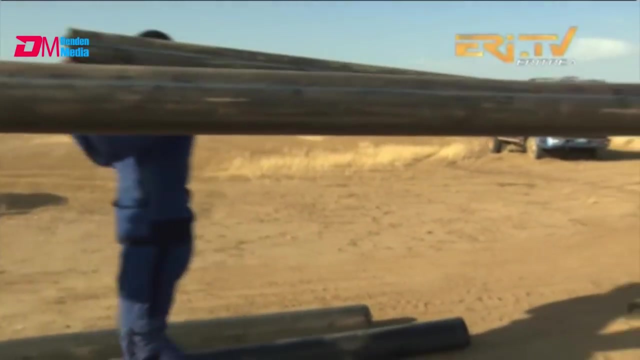 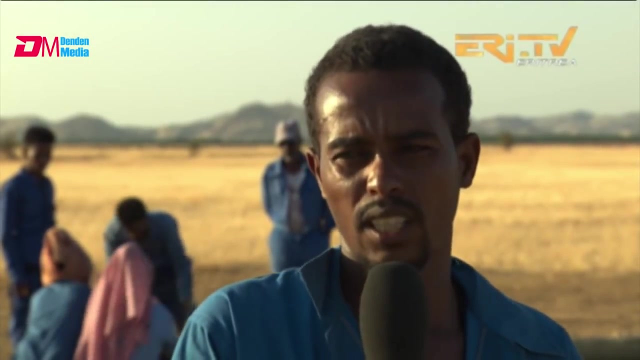 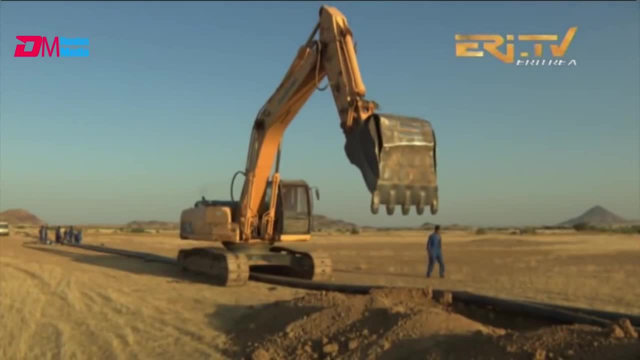 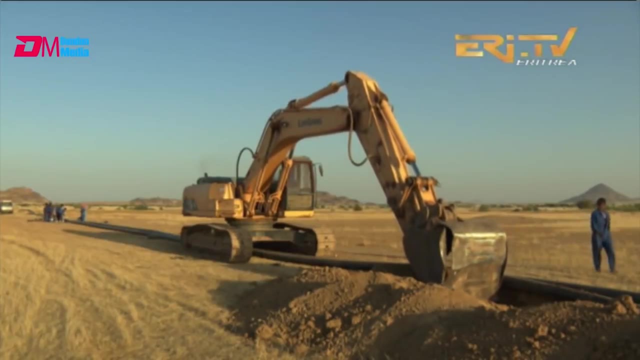 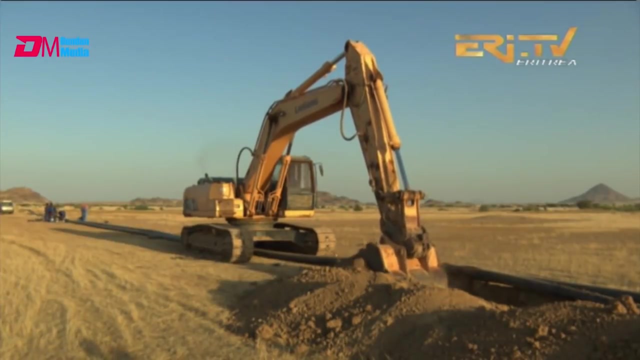 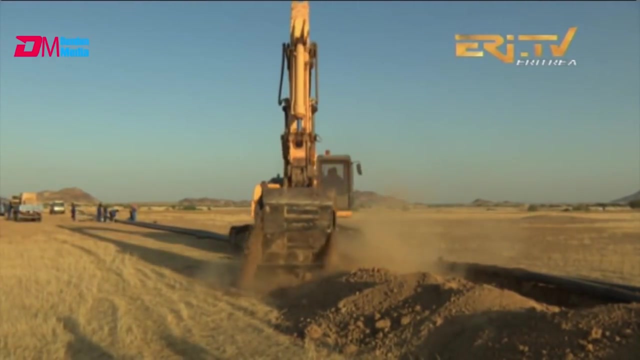 I am very happy to be here Camelot night with me. are by me, though it the condition of Allah. mr Wimpton Ocasio-Cortez, in Mufasa, busy well, had an abscess. the time you don't have to go. 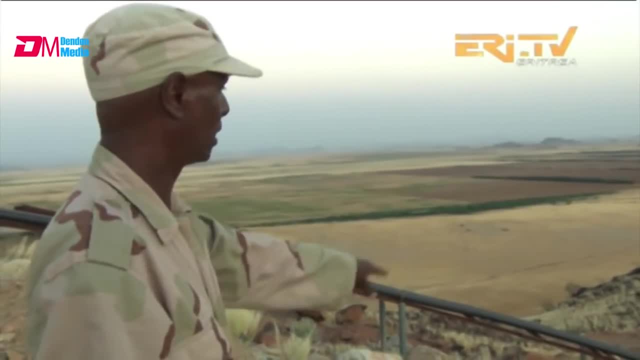 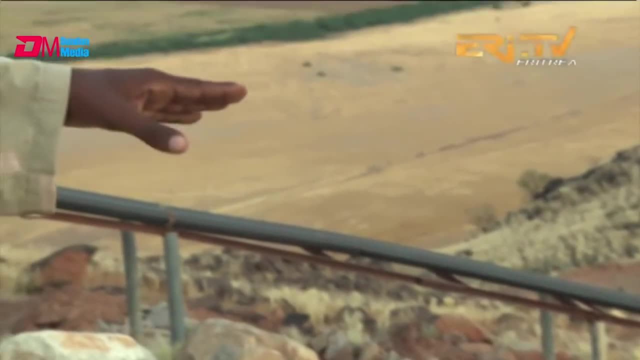 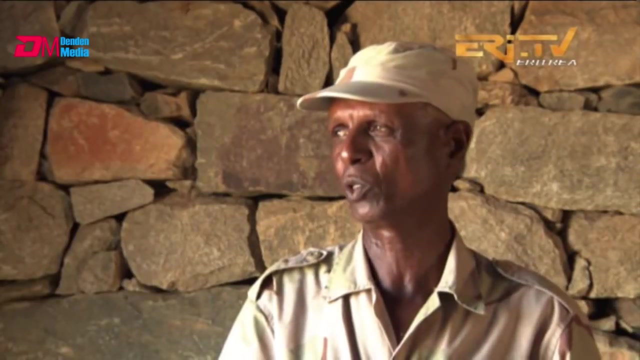 abisham on to a beat tanker at in tezcala cab, avi de gana, bagana cabana, that the community is doing good and doing good for the community. When I first came here I had the family under a tanker. I saw a tanker. 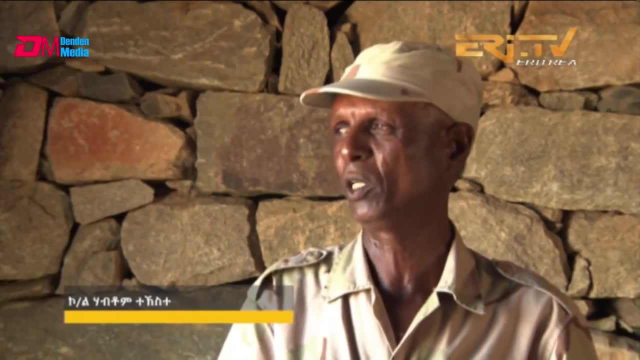 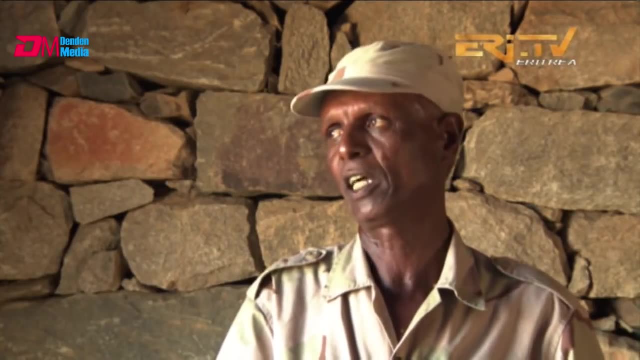 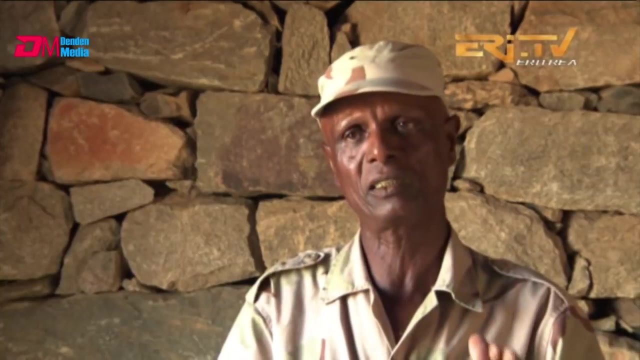 He had a flight of about 2,500 feet. I felt that the water was very pretty, I felt that the water was flowing. I wased that water. We then get the water from the village And then we get the water from the side of the river. 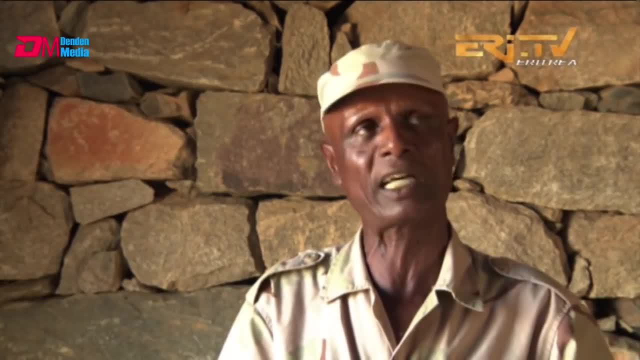 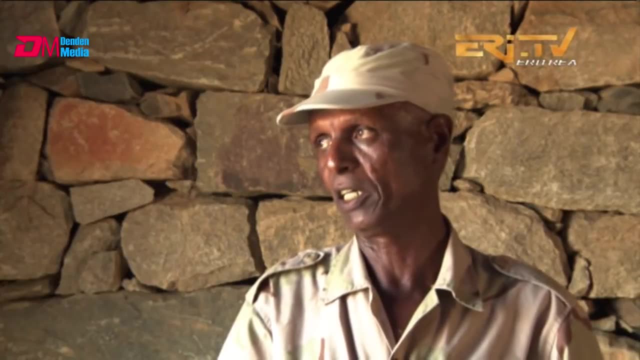 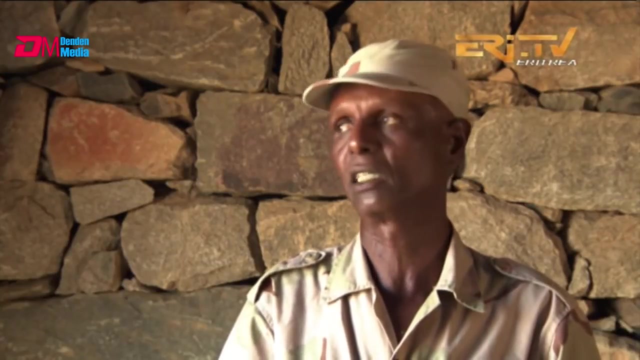 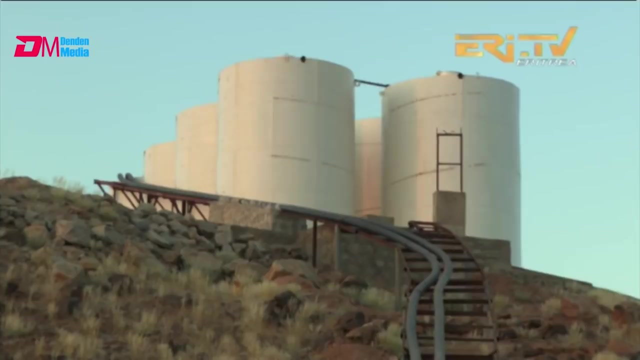 We then get the water from the river. We do this in the morning And then we cover the water with the mud. We also make the water from the river. I went to see my grandmother who was in the hospital. I was worried about her. 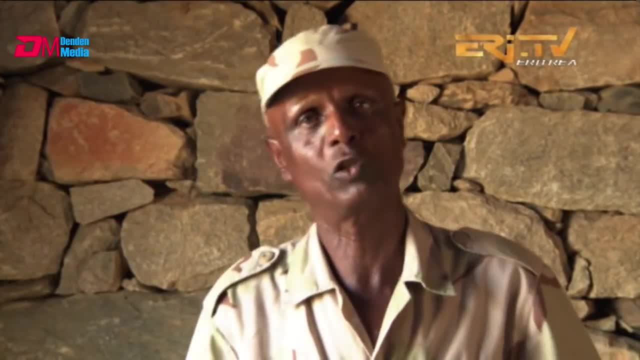 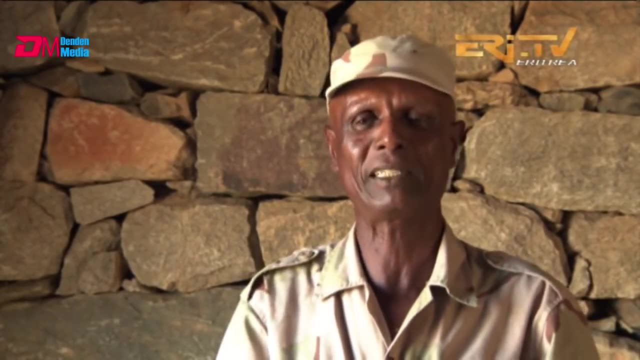 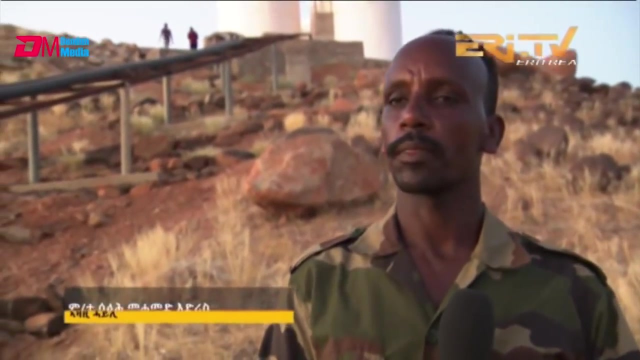 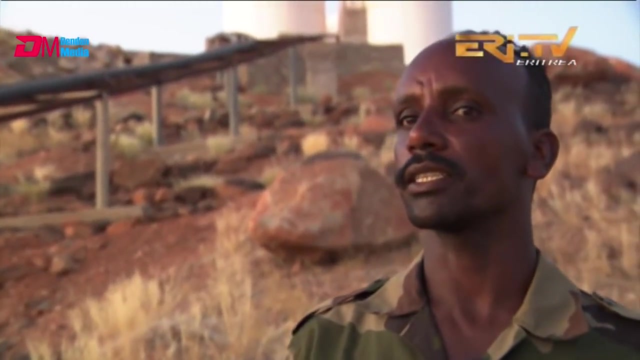 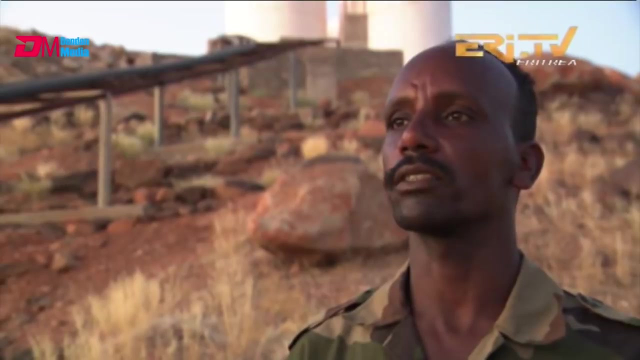 I told her not to go to the hospital. I told her that she will be safe. I told her not to go to the hospital. I told her that I would go to the hospital if I was to leave. Therefore, we have to teach them more and give them better education. 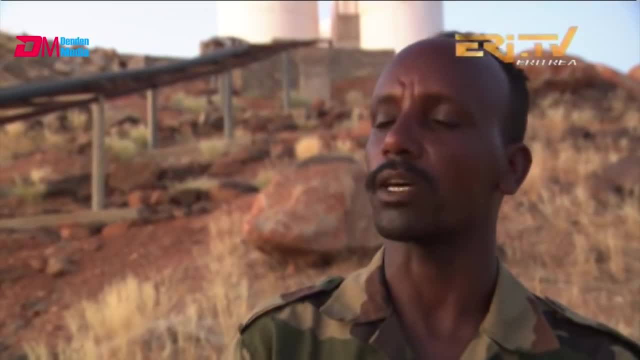 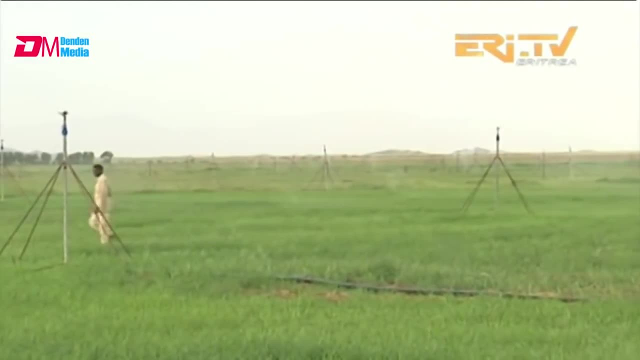 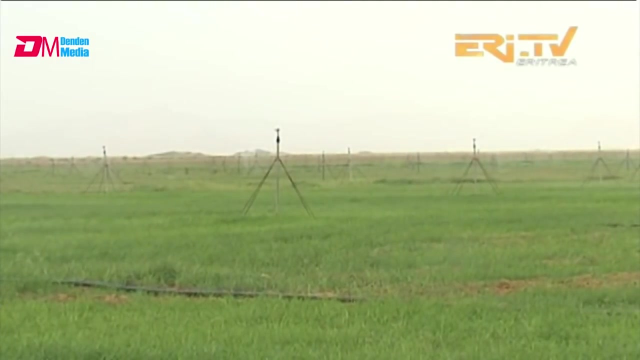 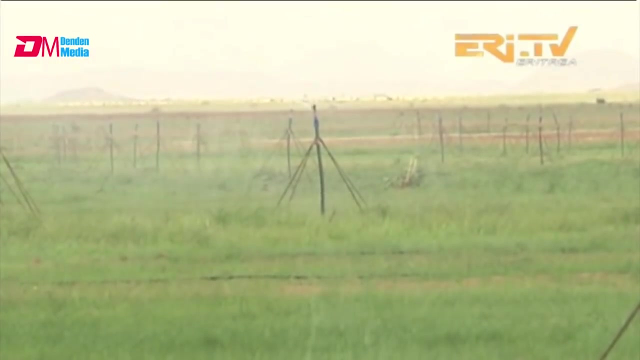 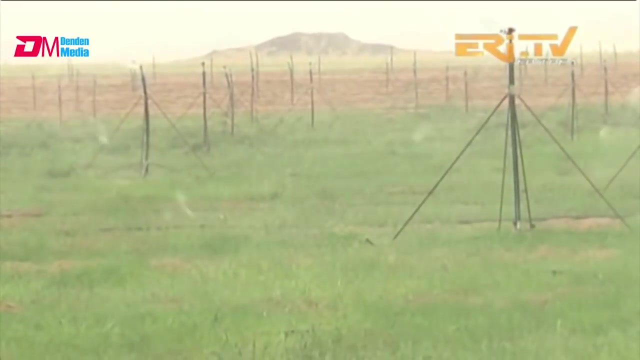 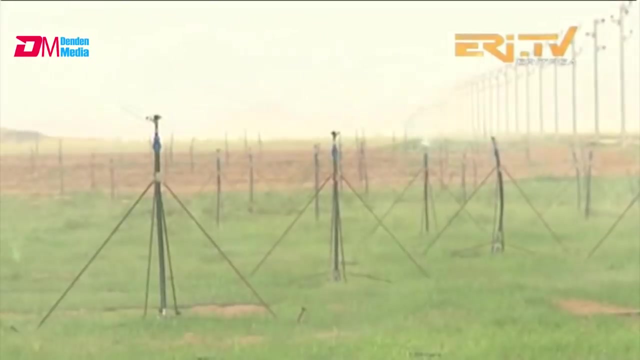 They will not be able to go to school and get better education. We have to teach them more and give them better education so that they can study well. The. The risk of being hit is high. Our people are affected by the water, and the water is very hot. 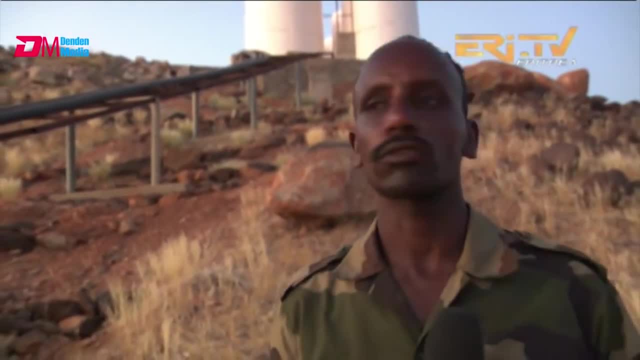 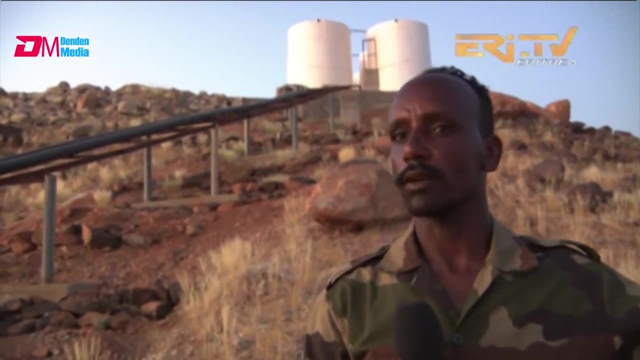 We are not very careful. That is why we had to avoid the water for the most part. We have to be careful, but we are not afraid and we are not afraid. We are not afraid of the water, We are not afraid to die. 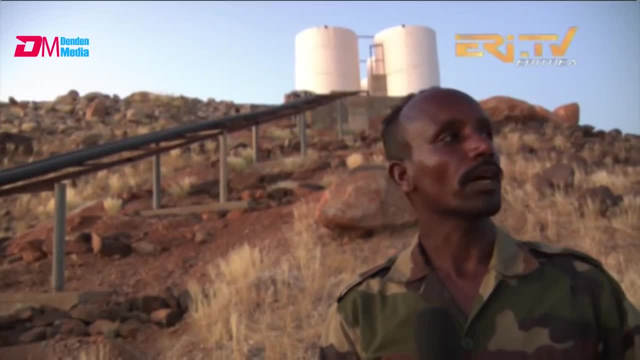 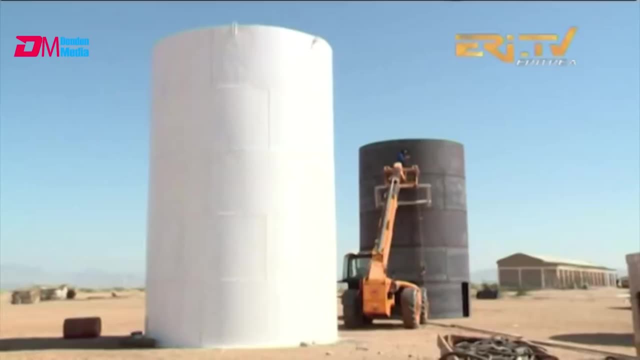 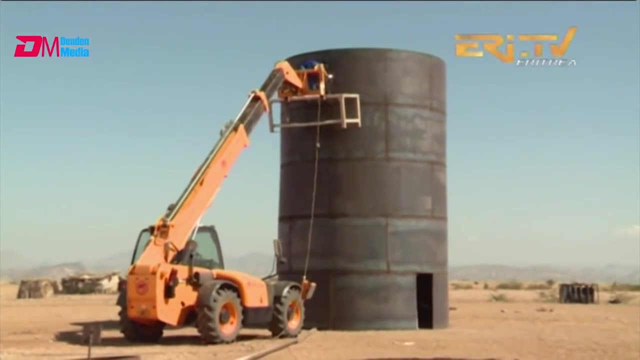 We are not afraid of the water. It could be that you want to be a master, but you don't have a job. You have to find a job. You have to have a job. We have to find jobs, We have to work. 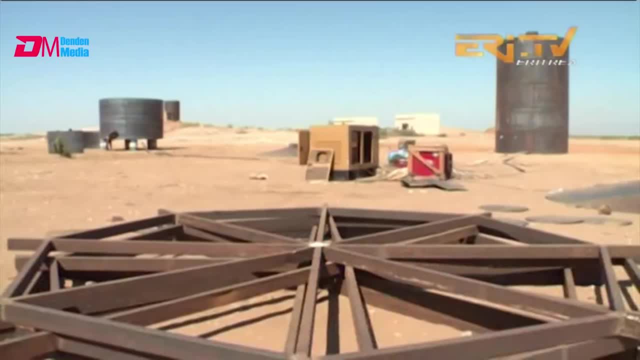 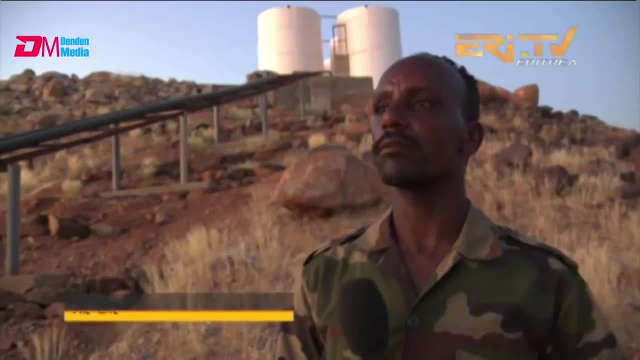 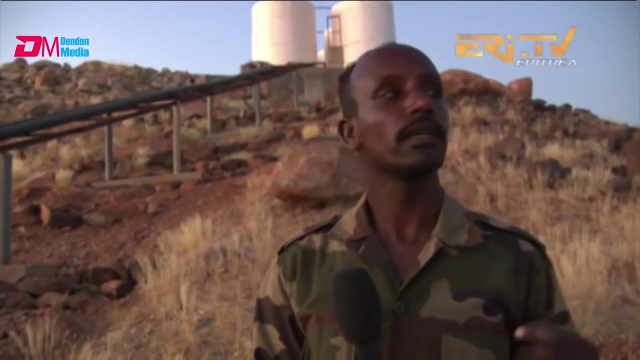 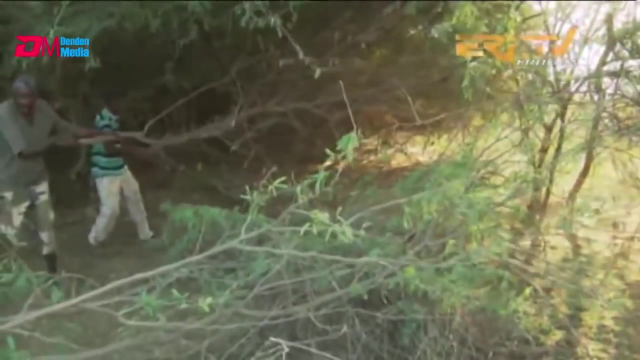 We must find jobs. We have to find jobs for the future generation. The older we get, the older we become. We need to be careful about the weather. The weather is not clear and ice is also not cheap. It is a very cold, cold weather. 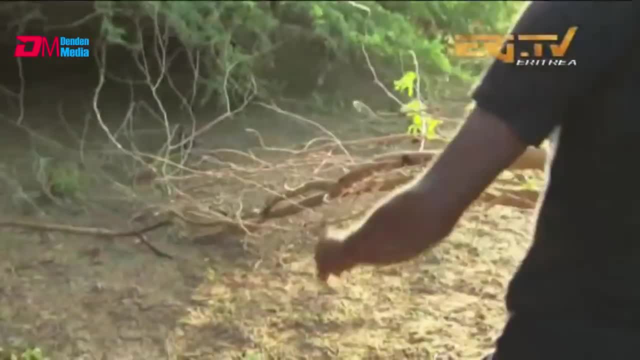 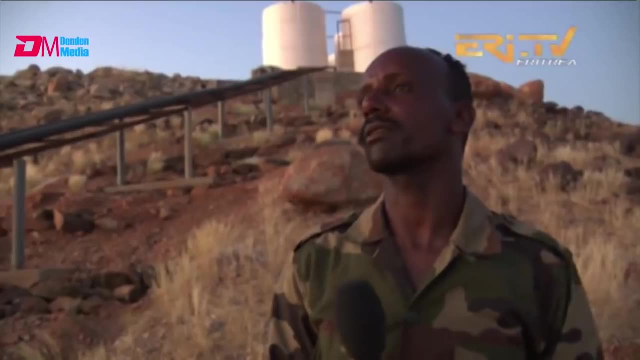 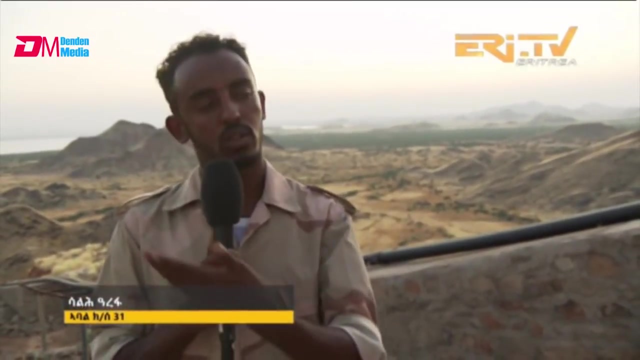 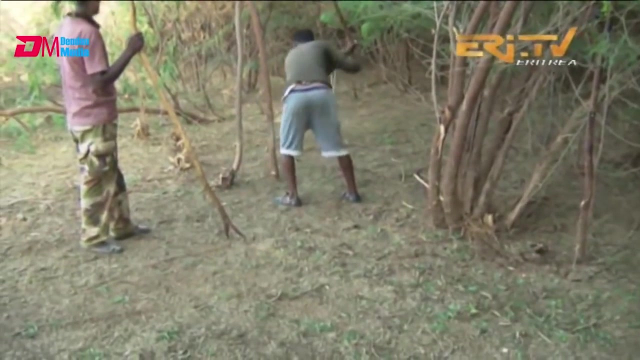 When it comes to the winter, I feel hot. It's very cold. It's cold and cold. I'm used to being cold. According to the government, there is no service to the residents of this area. We were not able to go. 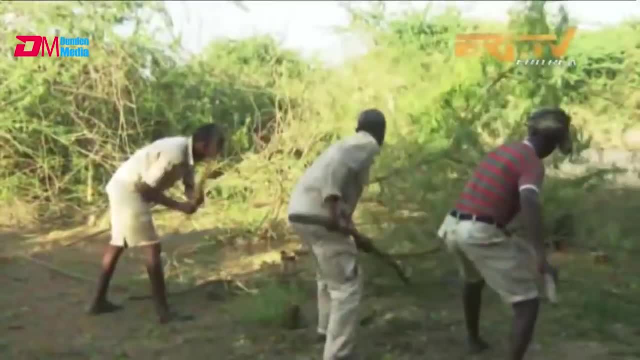 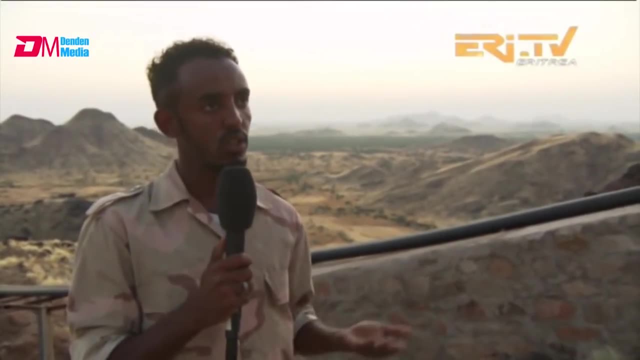 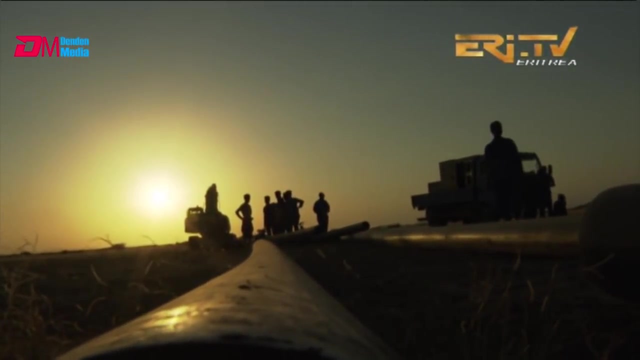 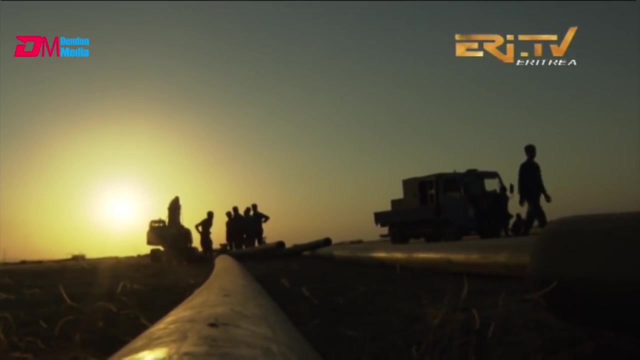 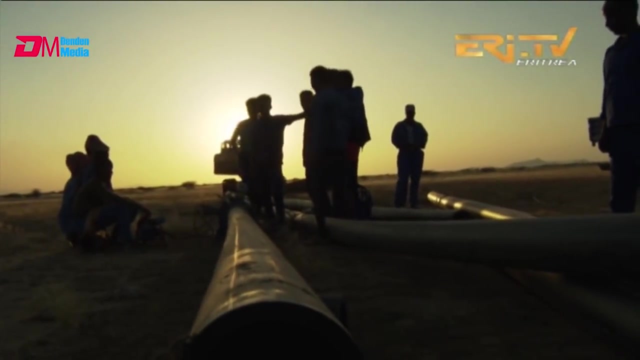 We left this place because we needed to save our lives. Otherwise, our lives would not be saved. In this video, I will show you how to make a very accurate and clean photo of your child. This photo is taken from a 4.7 km long photo. 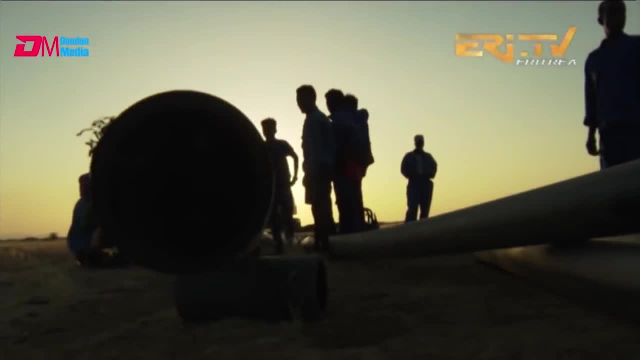 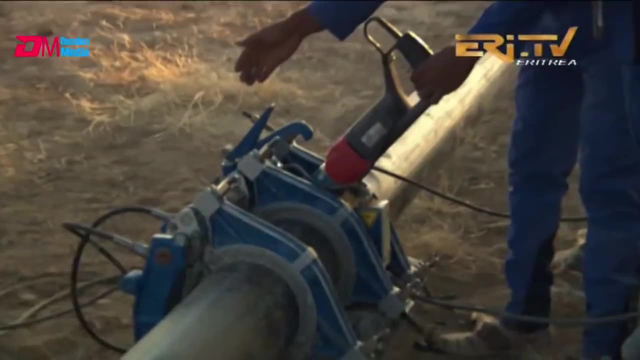 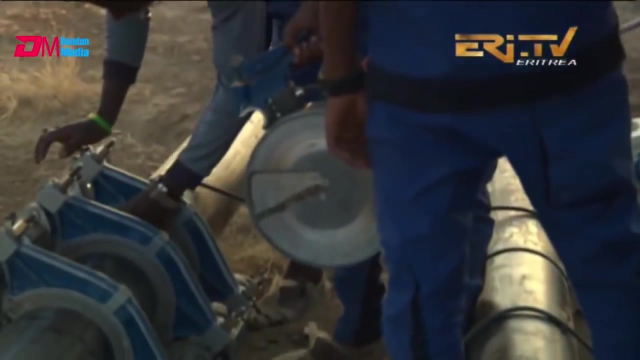 The size of the photo is 325 mm. I will show you how to make a very accurate photo of your child. The 90 PE plastic can be used for any type of work. We have been working on this project for a long time. 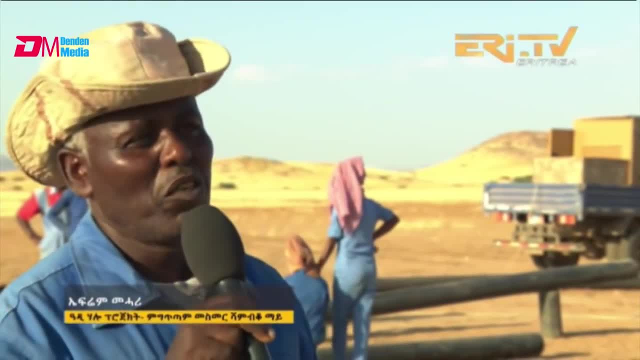 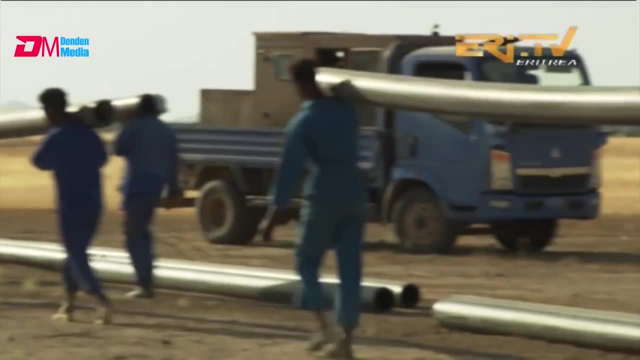 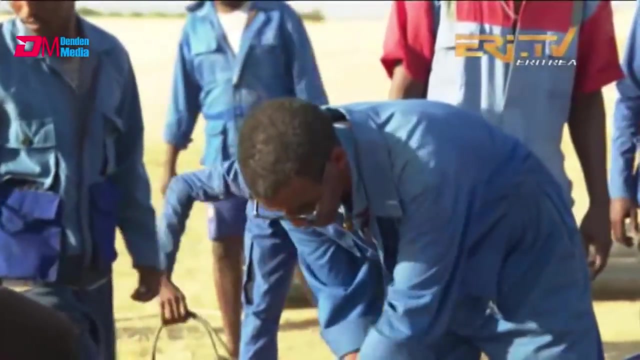 We have been working on it for a long time. We have been working on it for a long time. We have been working on it for a long time From the installed tools we received from the indentification group, From the lime больш. we have been working on it for a long time. 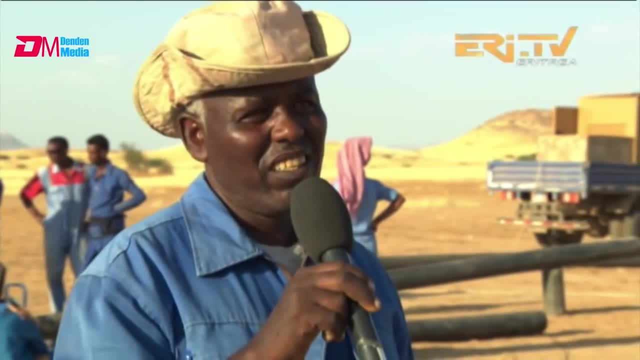 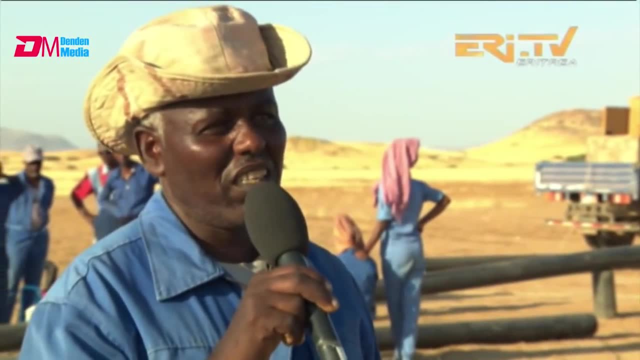 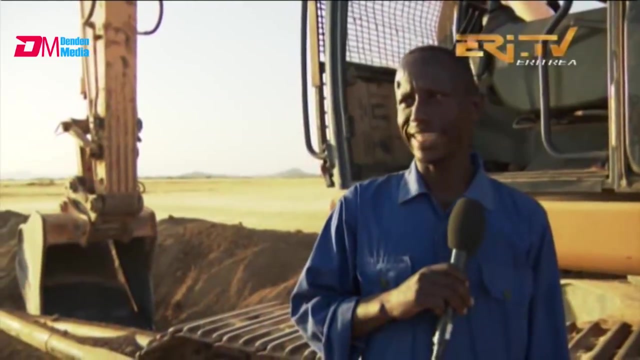 From the installed tools we received from the indentification group. We have been working on it for 13 kms: وحجات تمثالacking. We are also working on a waste restoration project. We are currently working in MNC. We are currently working in MNC. 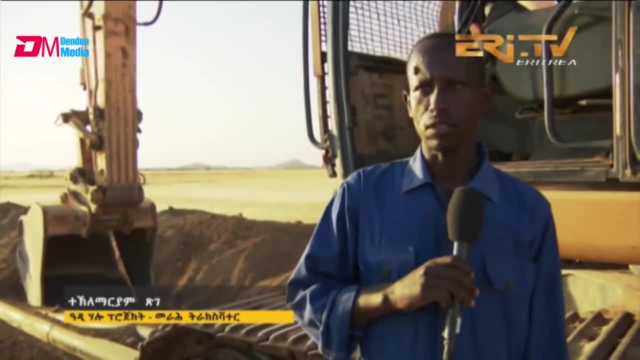 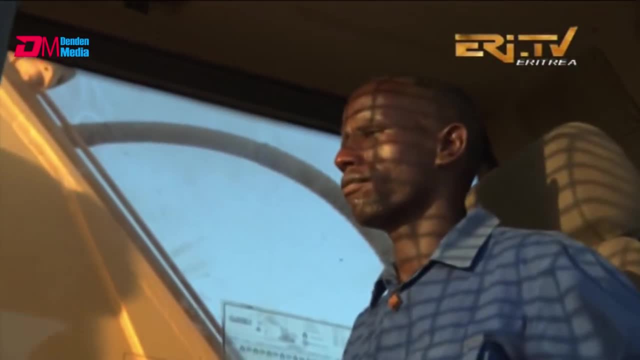 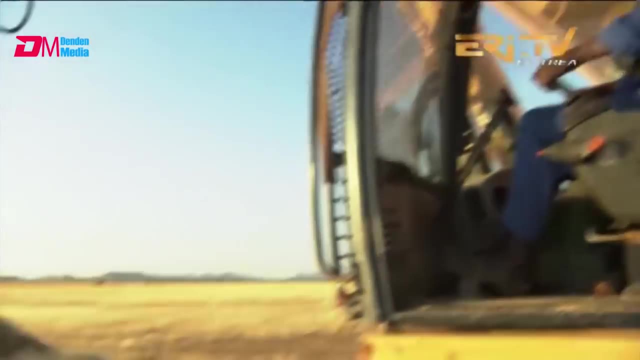 We are currently working in MNC and they can come back and fight. I'm very happy that we're free to fight. We're not fighting over the land, We're fighting for the land, and that's why we're fighting for our rights. 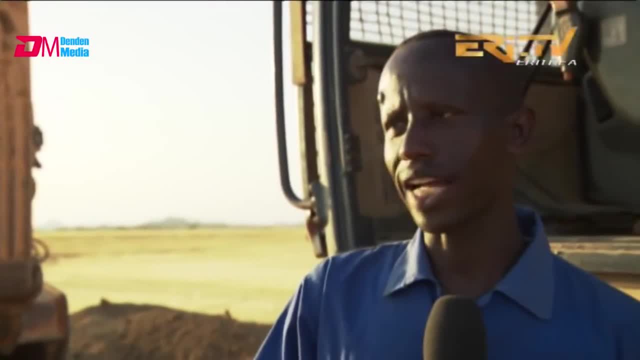 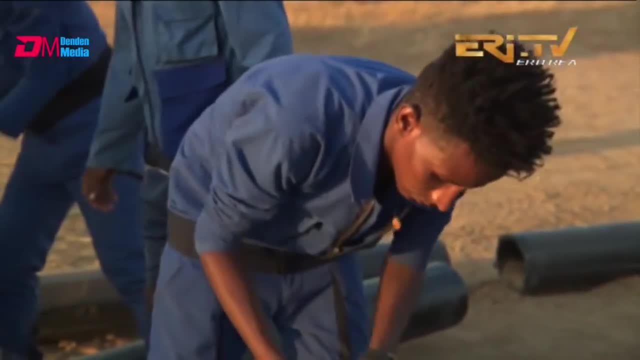 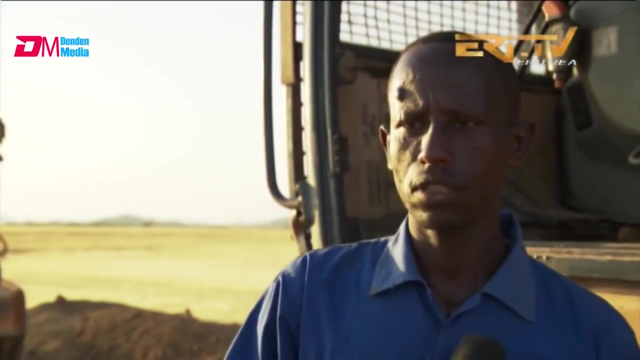 We're not fighting over the land. The river soaks up to up to 1.5 meters. The other side is about 1 meter deep And here there is a distance of just 1 meter. And if the length of that distance is 1 kilometer, 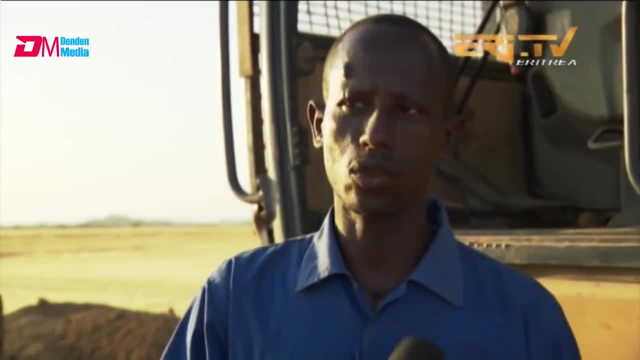 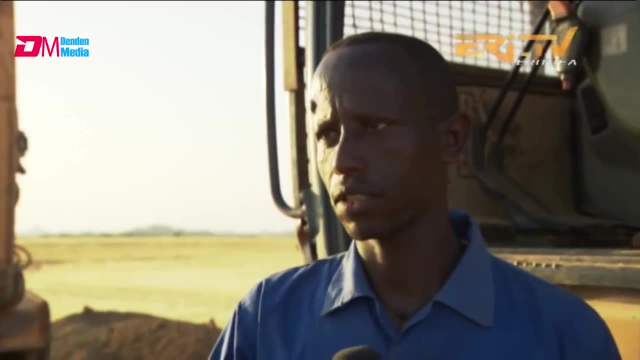 it will be 1.25 kilometers long. So if I stay on the road I can get 1.25 kilometers back. For example, if I go up there, I can get 4-15 kilometers. They have to be made in a new way. 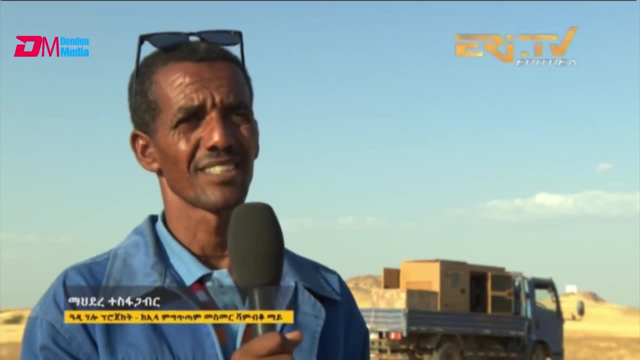 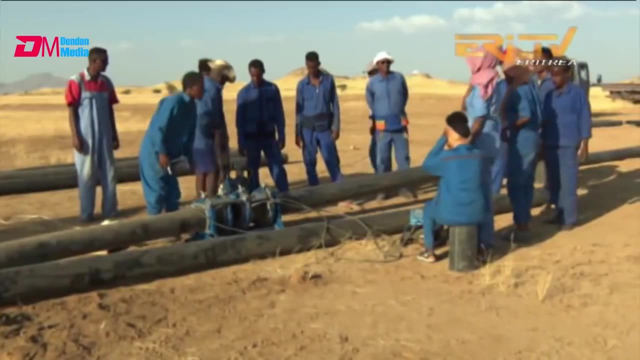 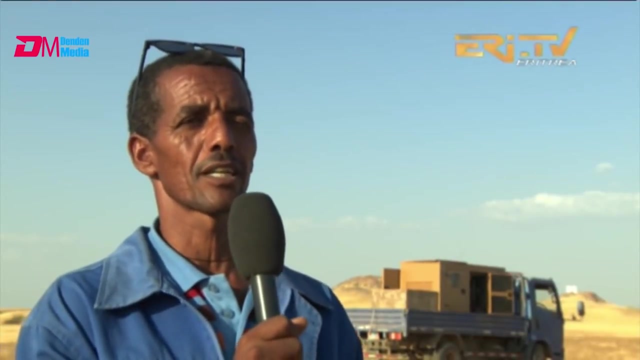 the same as the one they make now, and then they come in the new way and they are made in a new way. When they are made in a new way, they are made in a different way and they are made in millimetres. 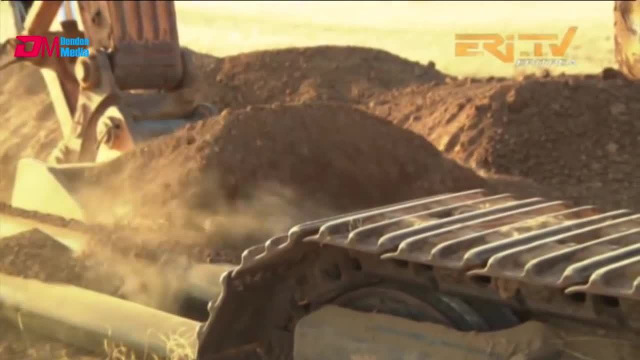 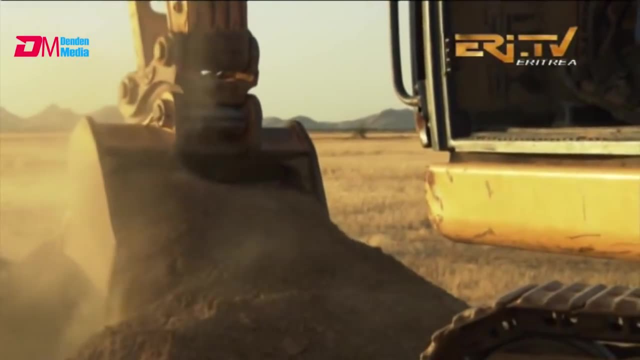 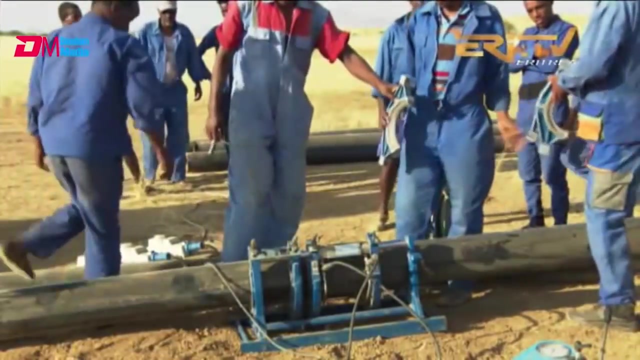 and then there is no need for other materials anymore. The project that will be launched in the city of Drabileko will be a project that will be a symbol of the future of the Nuneom community. The majority of the population of the Nuneom community are women. 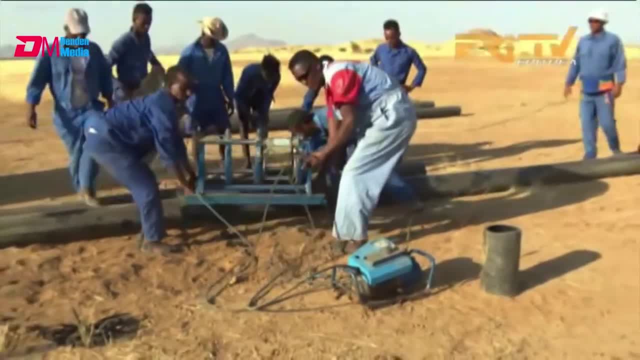 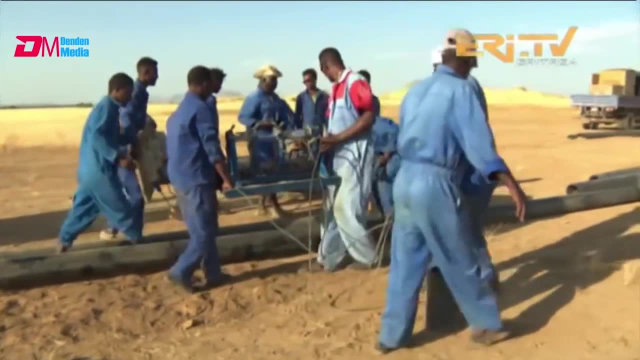 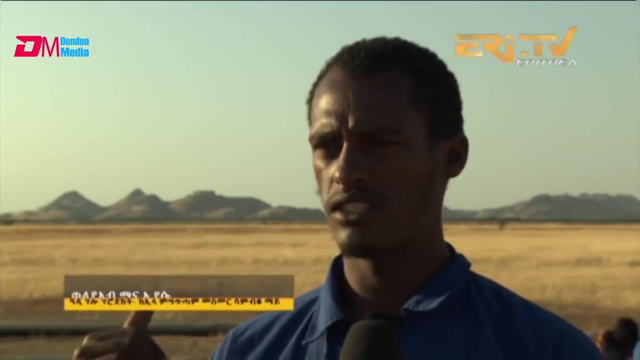 The government will be able to provide services to women. The project will also be a place for women to come and be part of the community. The project will be a place for women to come and be part of the community. I completed my first month of the job as a tucker. 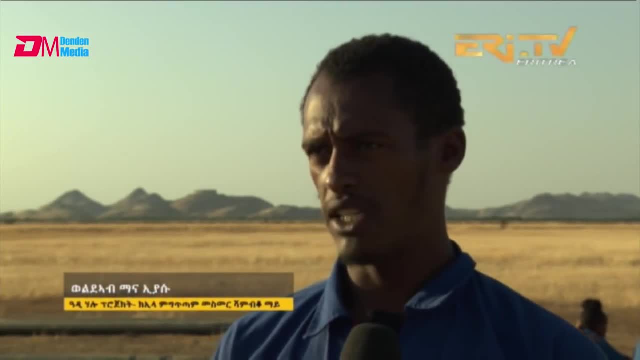 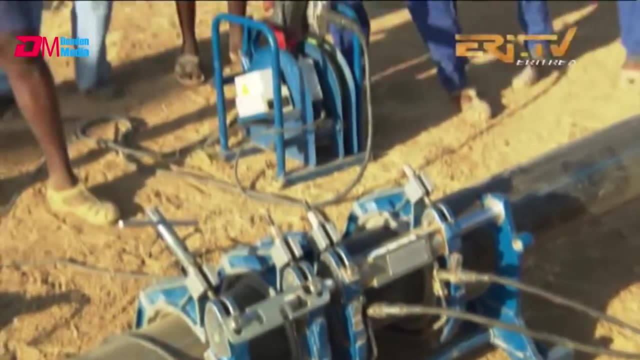 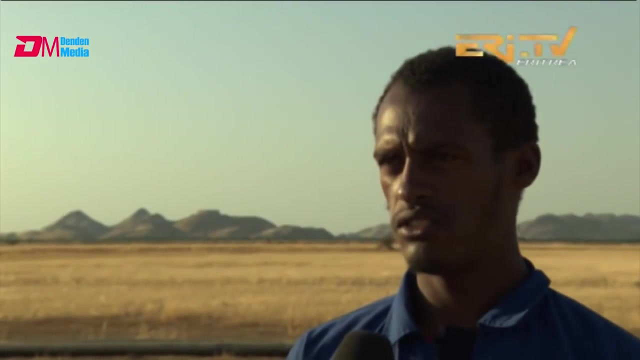 I use four water tanks and four water bottles to make a pot that can be used as a water tank. I then use a water tank to make a water tank and also use it for irrigation. I also work with a water tanker and a water Haharisha. 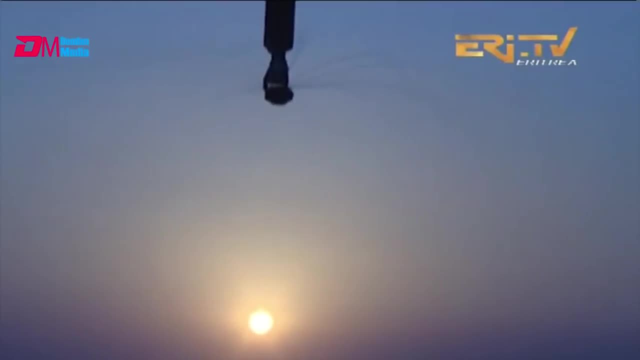 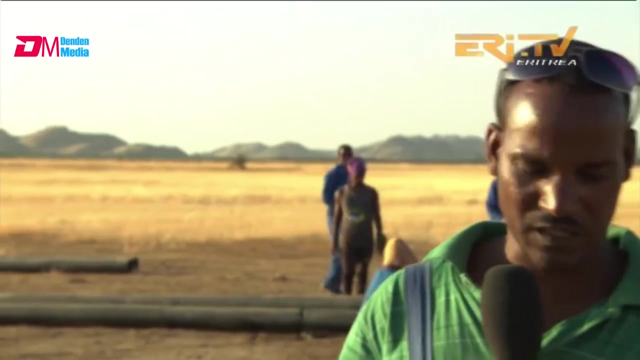 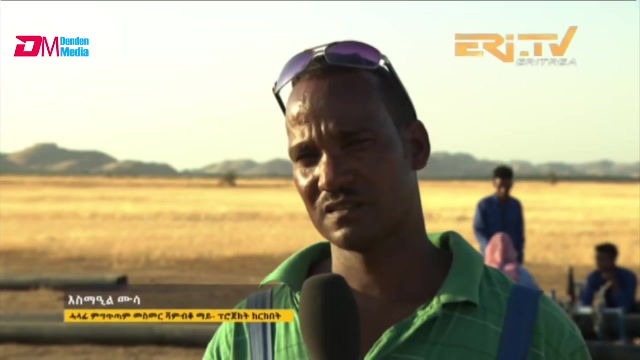 We have to irrigate the land, sprinkle it and then water it. This is how we get the water we need. The machines we use are made by our own hands. We don't use our hands. We use our hands. We use a pipe. 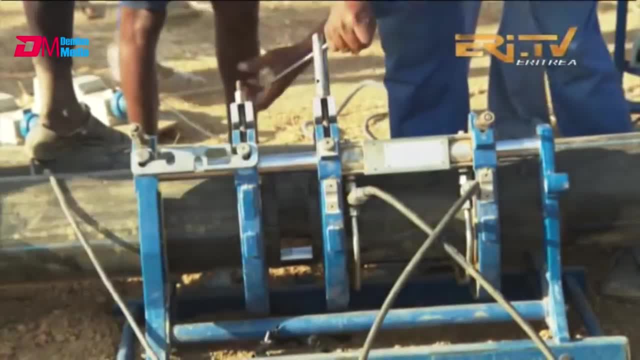 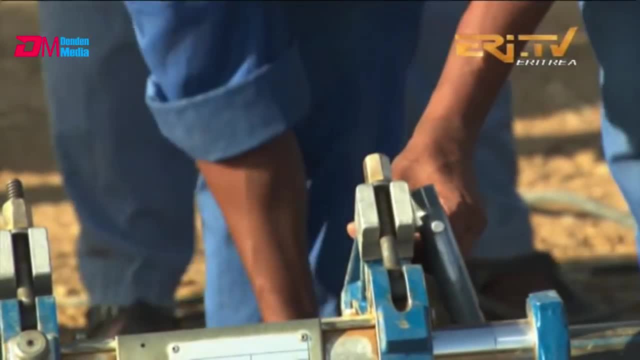 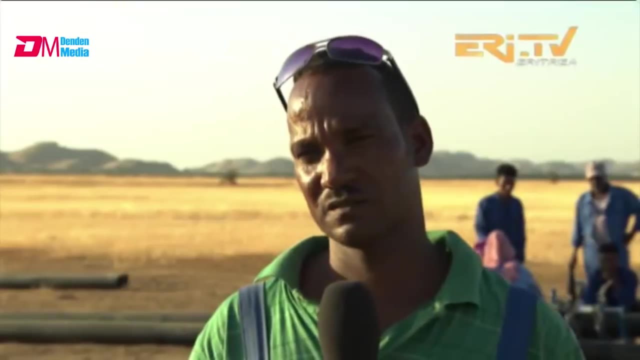 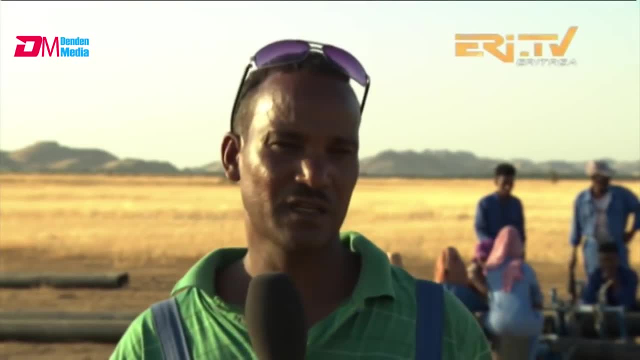 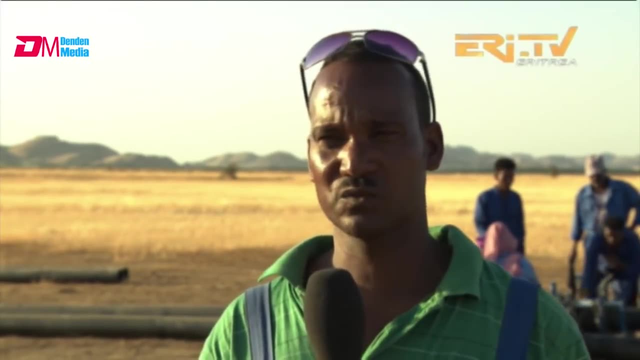 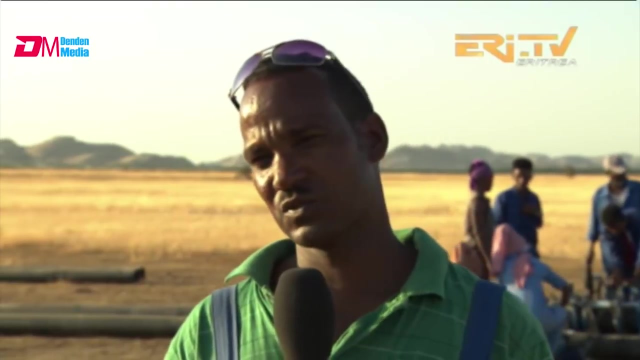 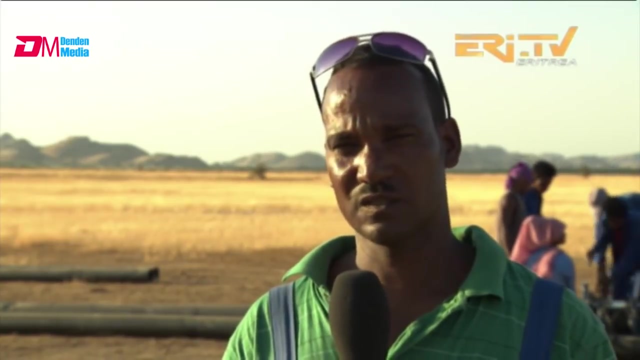 and then the houses got polluted In between. We produce thisEC and then we use it From this source. we prepare set crops and thank you. and we need to fight. We need to make sure our people don't die. We are still fighting. 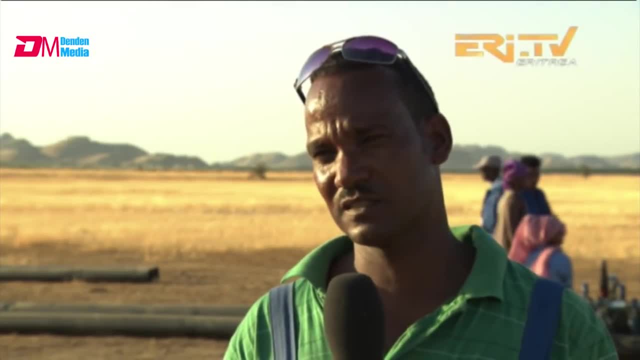 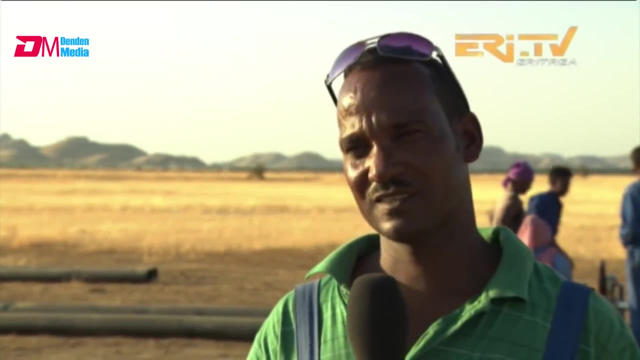 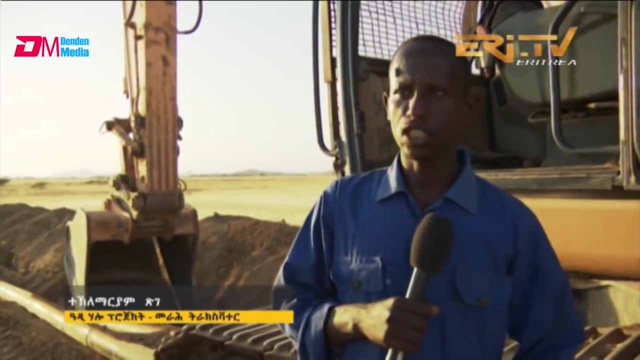 We have to fight for our people. We have to fight for our people. We are still fighting. We are not fighting for our people. So my brother and I were able to move all of these taul to the other side to make the saplings available right here. 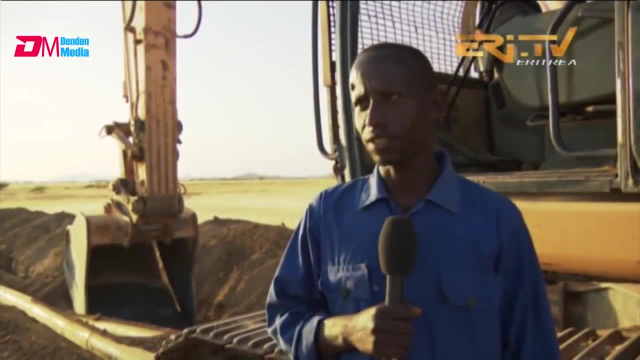 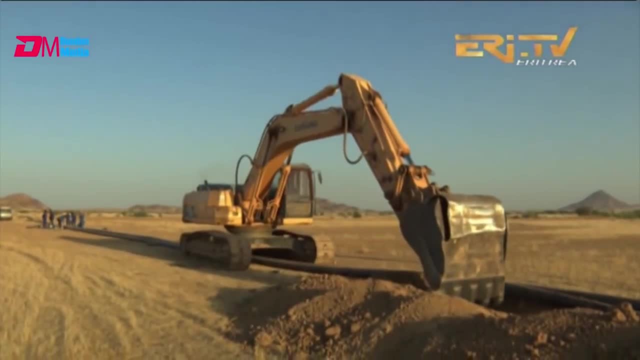 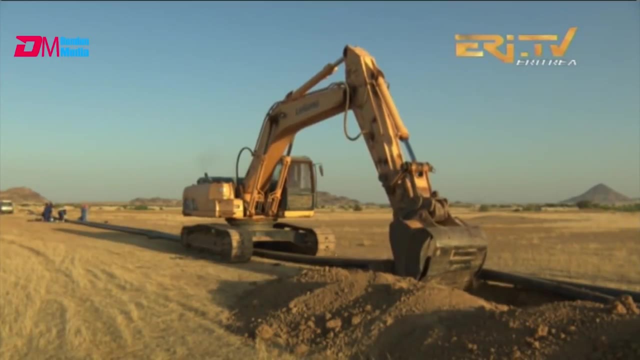 My brother had looked for a place to keep this and it was only to find a place to keep. these days, The water is running very fast and is very fast, But the water it flows fast and spends a lot of energy. 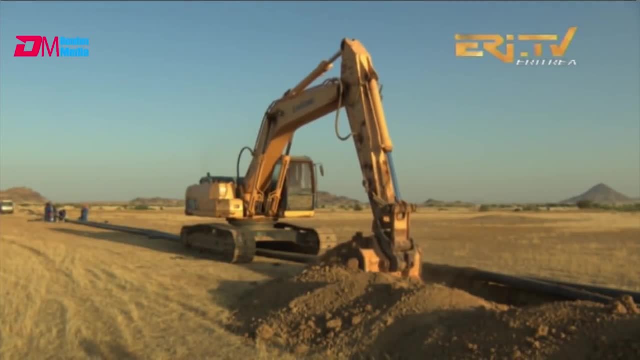 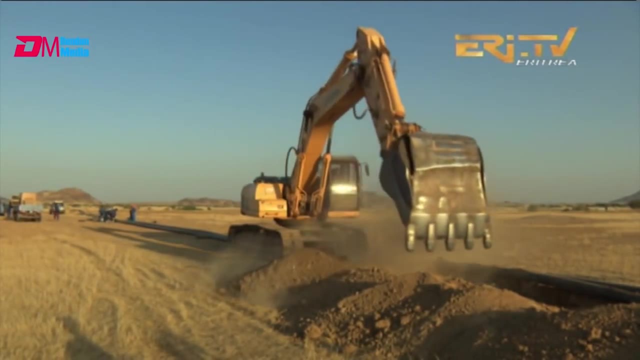 The woman who went to the grave was not a woman but a man. That's what we asked and we said: we will take her with us. but we need to take her with us so we can see if she is alive. 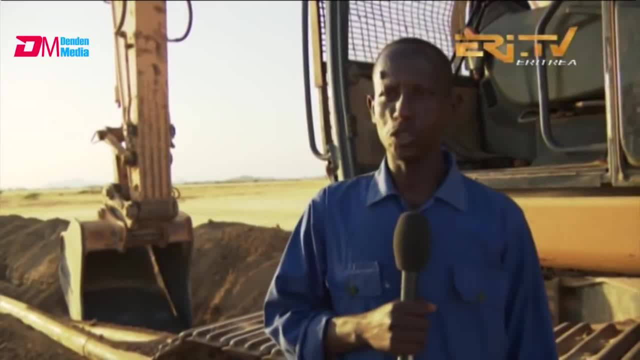 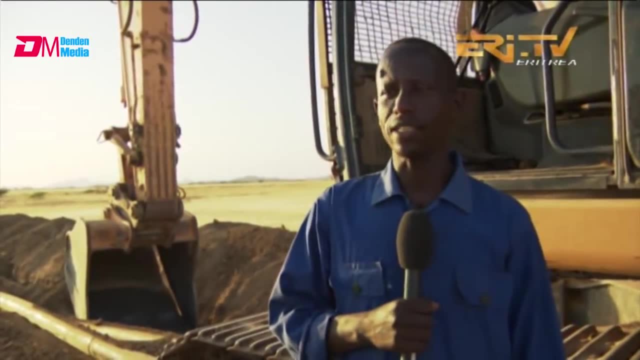 But we have to see if she is alive, Because if we don't know, we don't know. If we have no idea, we will not know. If we have no idea, we will never know, We will never know. We need to see if she is alive. 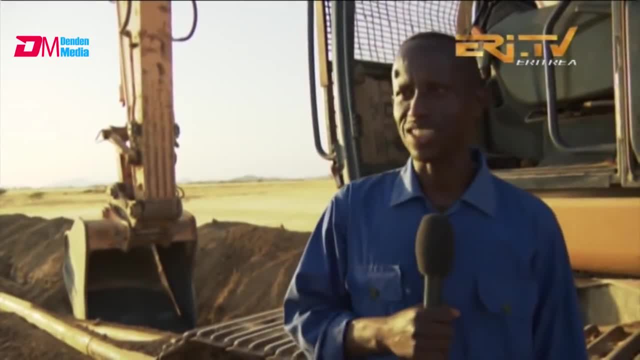 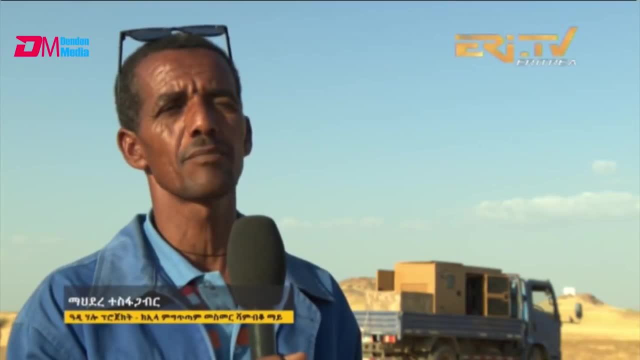 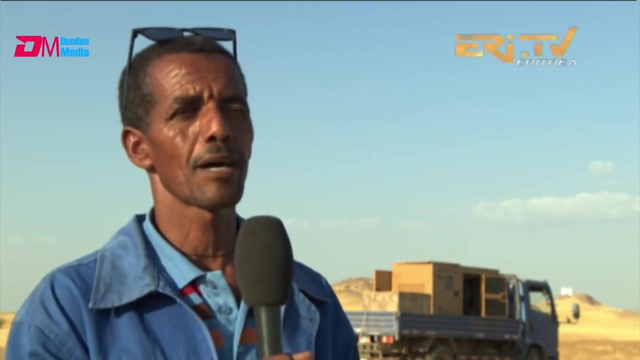 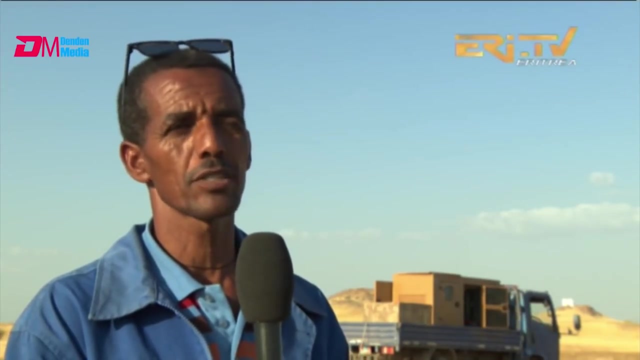 do the same as we're doing, everything will be fine In Zimbabwe. our people are very firm with us and we rely on them a lot. They come here to help us and support us. Their help will help us manage this In Zimbabwe's. people are very useful. 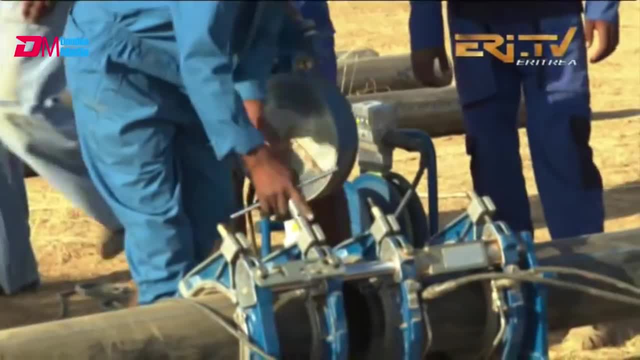 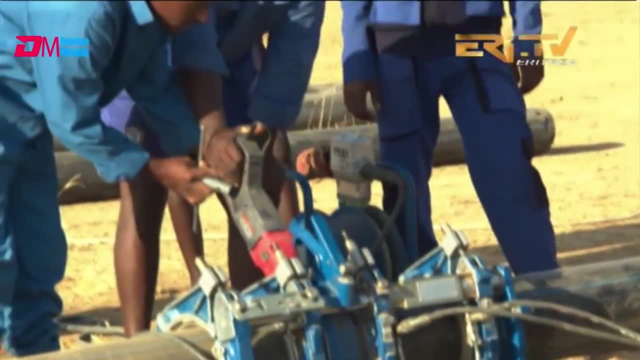 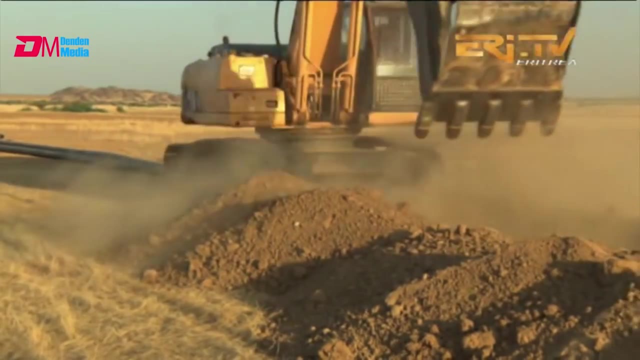 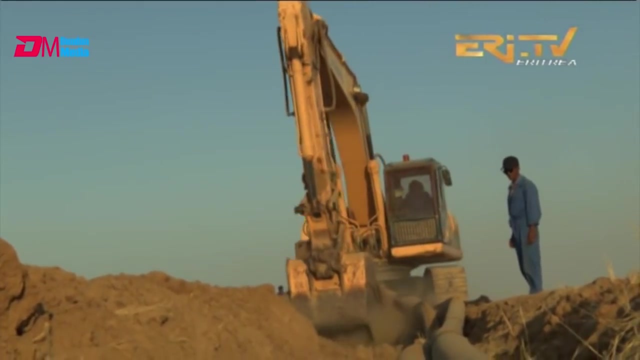 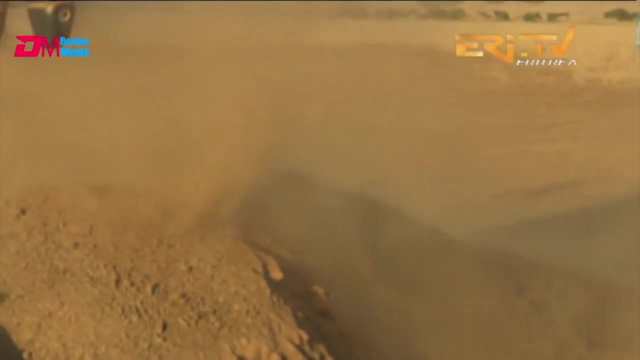 They make a living from us and support us. The speed of this machine is the same as the speed of an agro-industry machine, but it is not as fast as the speed of an agro-industry machine, but it is faster than the speed of. 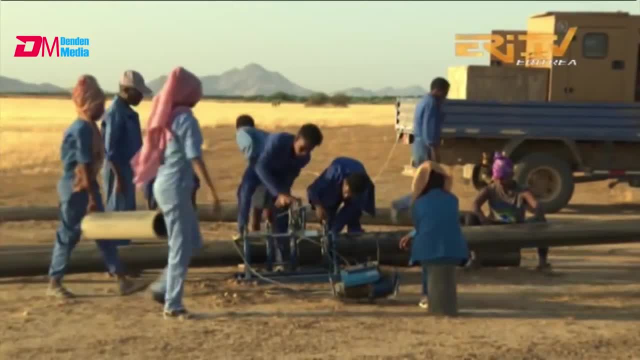 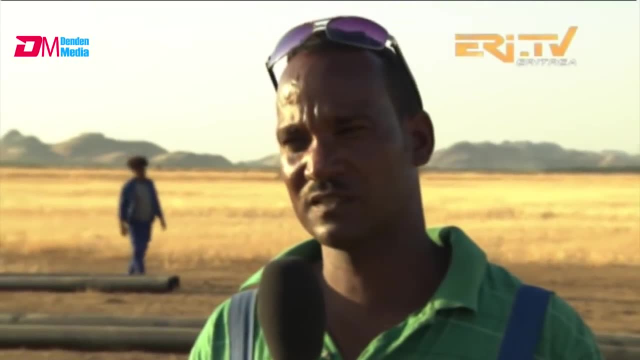 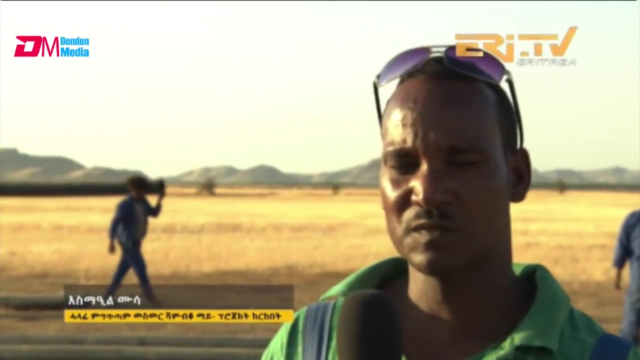 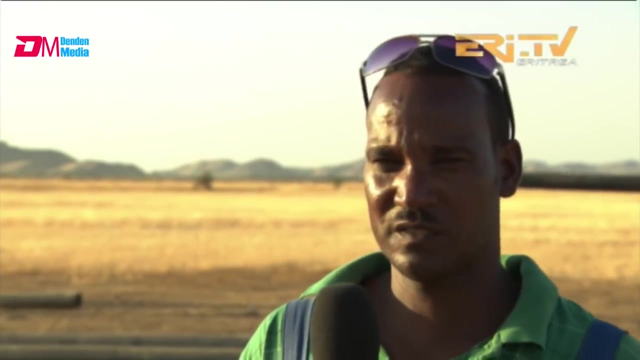 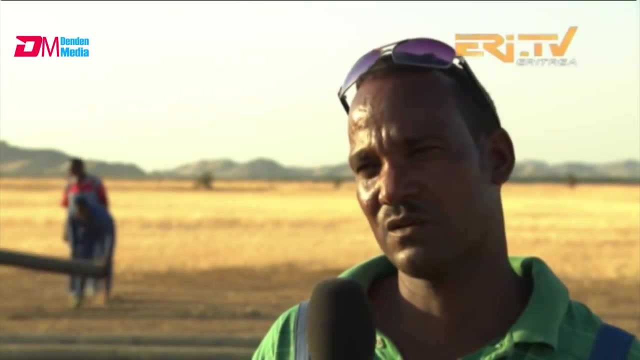 Abkar Aba Metsai Abimali Nsafiho Frenzahat Tmedb Srehka Iwadadalo, so that we can keep our business going and to be able to give back to the people who need it most. 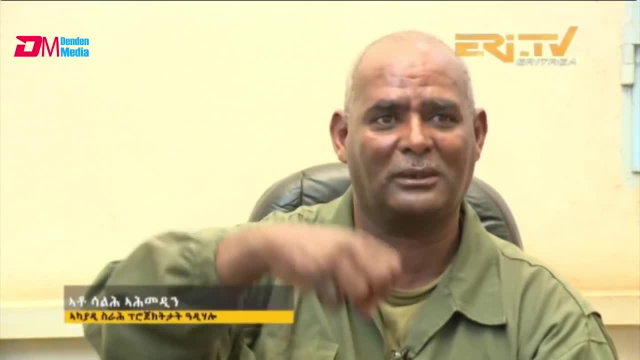 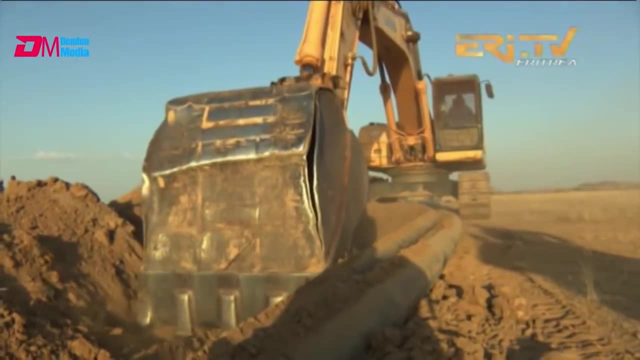 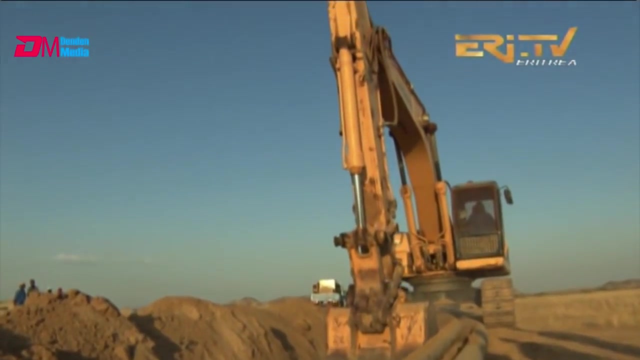 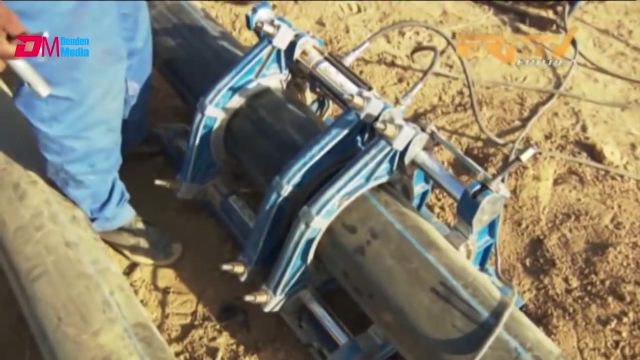 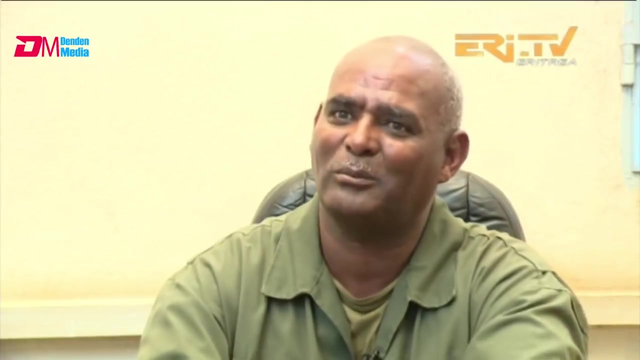 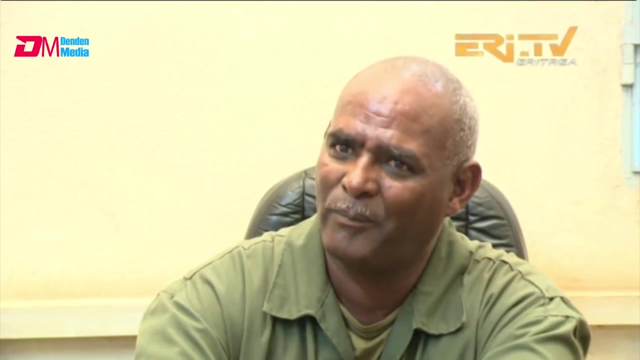 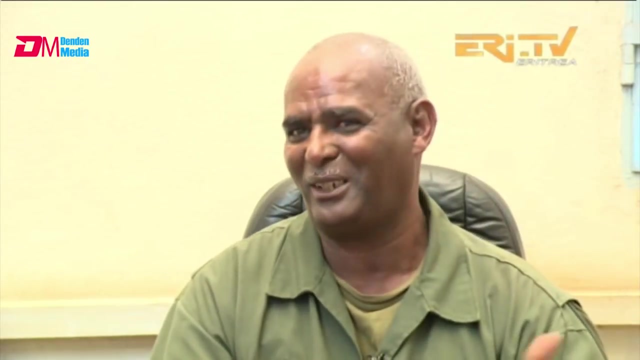 The issue now is not the people, It's the people who have to leave the city. The people who are left behind from the government are the ones who are the ones operating If you have to leave in AOT to Mursi Maledi.